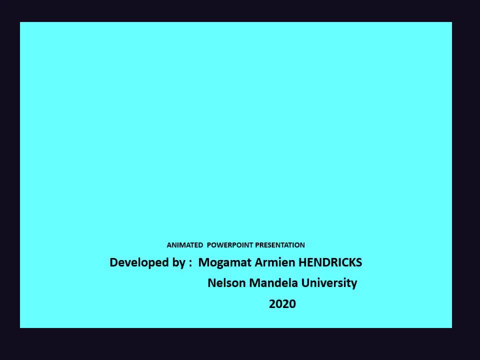 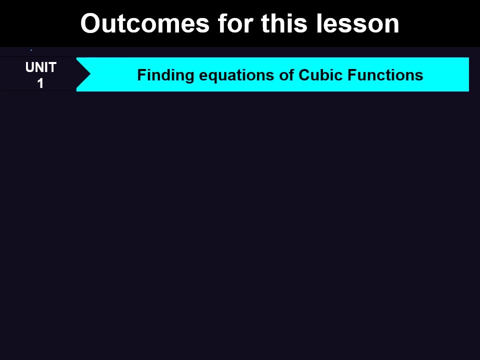 Hi, welcome back to Maths with Armin. This is part 4 of differential calculus and we're going to look at interpretations of graphs of cubic functions and, specifically, some inequality relationships. In this lesson we're going to first of all look at finding equation of cubic functions where the 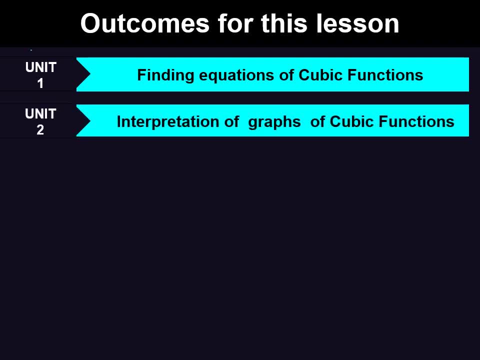 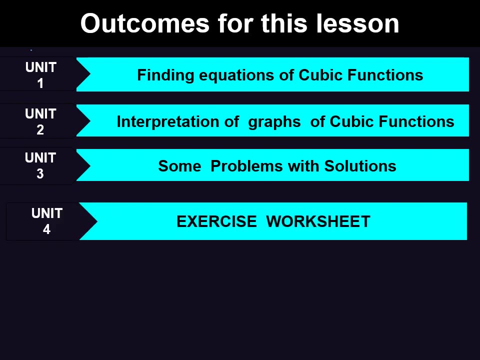 graphs are given. Then we're going to show you how we can interpret graphs of cubic functions and specifically some inequality relationships. Then we're going to do some problems with detailed solutions and, as usual, there will be an exercise worksheet for you to practice these concepts and 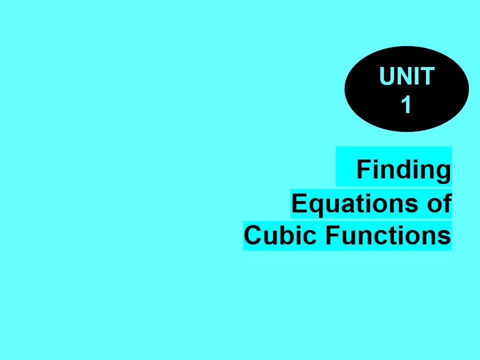 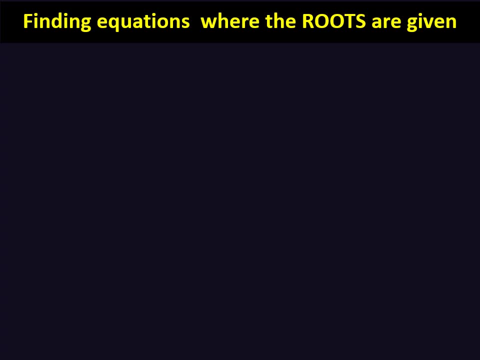 skills. Let's start with finding equations of some cubic functions. We're going to start off with finding equations of cubic functions where the roots are given Being a cubic function. this is the standard form of a cubic function. consists of four terms. I have a3, b2, c and d. 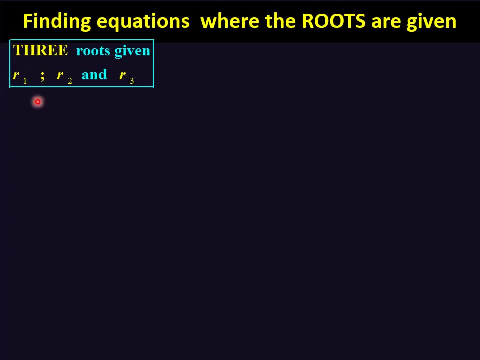 What's the maximum number of roots? That's right, three. So let's say we have there the three roots, r1, r2 and r3.. Let's look at it graphically. There we have a cubic function, There we have r1, and you can see. 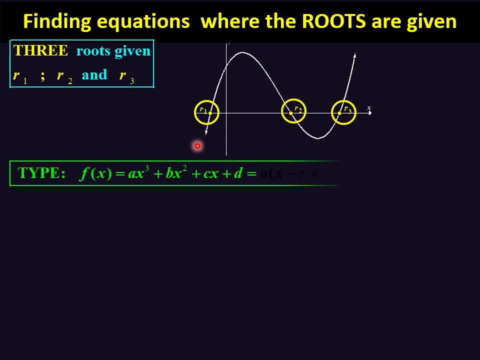 there's r2 and there's r3.. Being a cubic function, this is the standard form of a cubic function. It consists of four terms. I have a3, b2, c and d. Now, because I have a coefficient of a, I can have a, then x minus the 1 root, x minus the 2nd root, x minus the 3rd root. 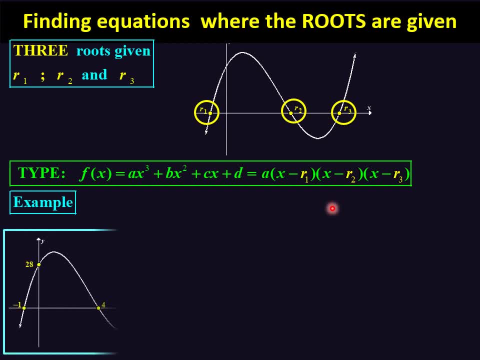 Let's look at an example Here. we have an example and let's see what is given. We have a root at negative 1,, we have a root at 4 and we have a root at 7.. So we can actually substitute these roots directly now. 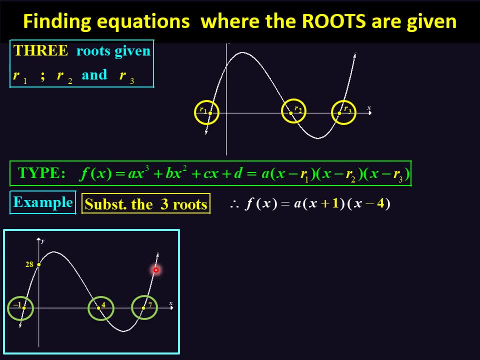 So if I substitute those roots, the first one, negative 1, becomes plus 1, positive 4 becomes negative 4 and positive 7 becomes negative 7.. But if we look there, there's another point, that's given the y-intercept 0 and 28.. 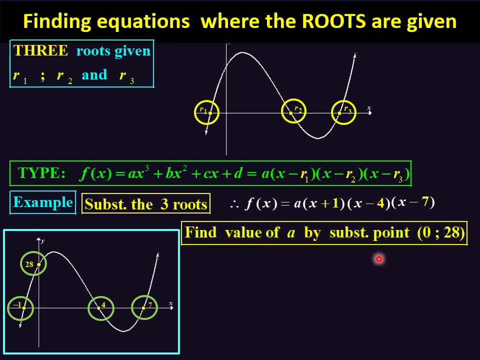 Now, if we substitute 0 and 28,. x is equal to 0, and what will be 28?? That's right, the fx. So if I substitute the 0., 0 and fx, now is 28.. And if we calculate that, you know that's negative 4 times negative, 7 is 28.. 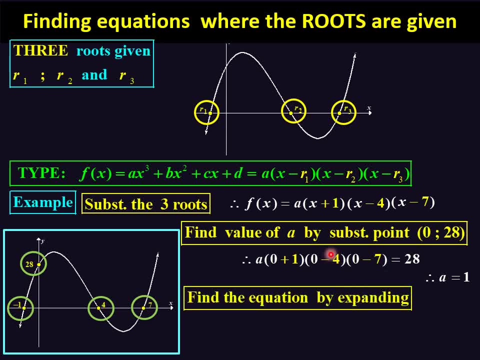 28a equal to 28.. It's very simple: a is equal to 1.. Now I now substitute a as a 1 and I'm going back to my fx now. So a is a 1, I'll have x plus 1.. 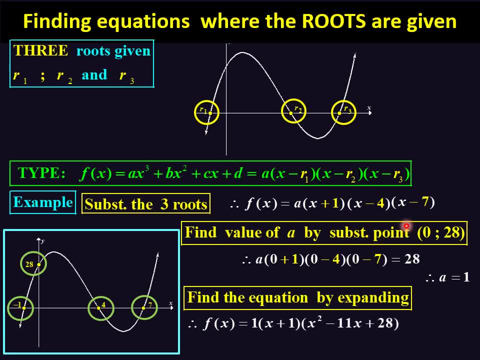 To expand that. it's advisable to expand by taking The last two brackets first. expand them, then I end up with x squared negative 11x and plus 28. And then you can expand that further. Maybe you can do it in an additional step. 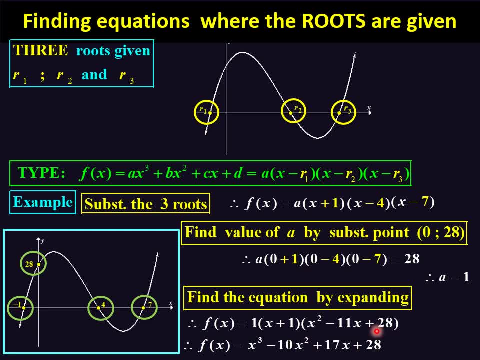 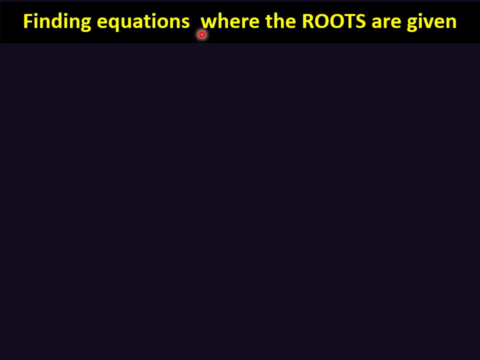 And the final part. there would be x cubed minus 10x squared plus 17x plus 28.. And there we found the equation here. Let's look at the following situation Here, where the roots are given, but in this case only two roots are given. 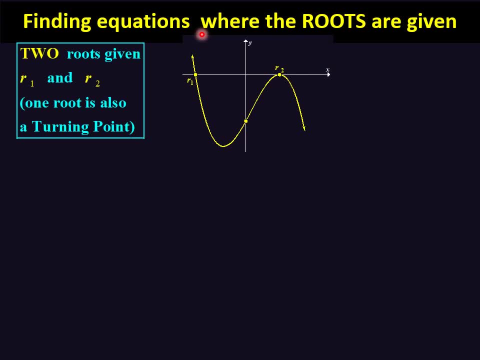 One of the roots is a turning point. There's the one root, r1, and there's the other root, r2.. Now notice: r2 here is a turning point. That means that these we have equal roots at that particular point there. So that's the form of the cubic equation. 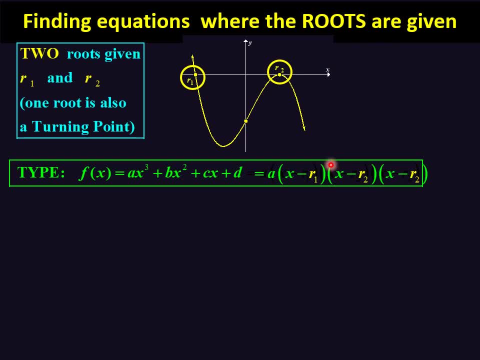 Let's insert the first root: x minus r1.. x minus That's r2.. As you can see, the r2 is the one that's going to be repeated. Let's look at an example. What is the first root? 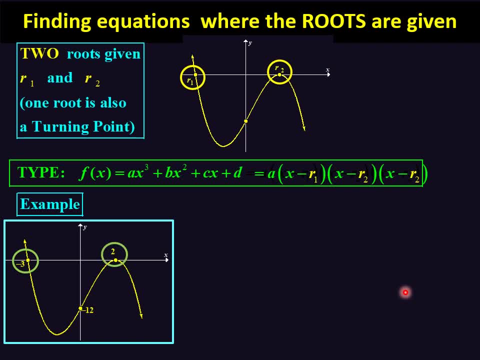 Negative: 3. And the repeated one? 2. See, the repeated one is the one that is associated with either a local maximum or a local minimum. There's the y-intercept, So let's substitute the two given roots, So that's going to be x plus 3.. 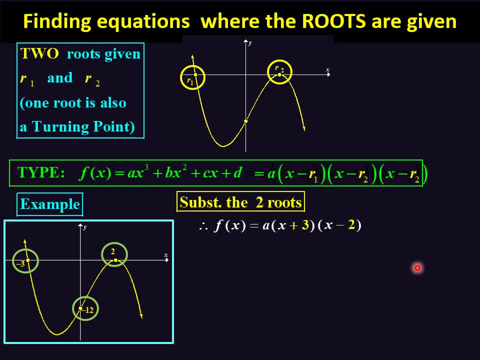 The other one is x minus 2.. And it's the x minus 2 that is going to be repeated. Now we have to find the value of a. That we can do by substituting the other points 0 and negative 12.. 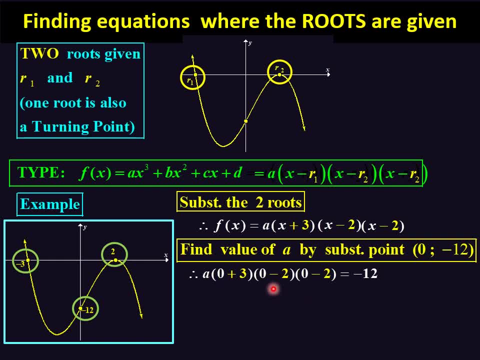 Substitute that We end up here with. That gives us 12a equal to negative 12. So a is negative 1.. Now we can substitute the negative 1 back into that expression And we multiply these two factors, the second two factors there. 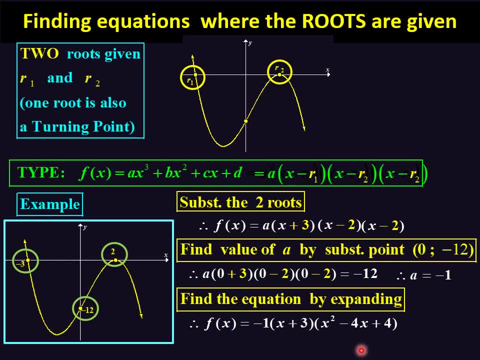 And we expand that, There's the. We end up with x squared minus 4x plus 4.. And if we remove all of that here, we end up with negative x cubed plus x squared plus 8x minus 12.. 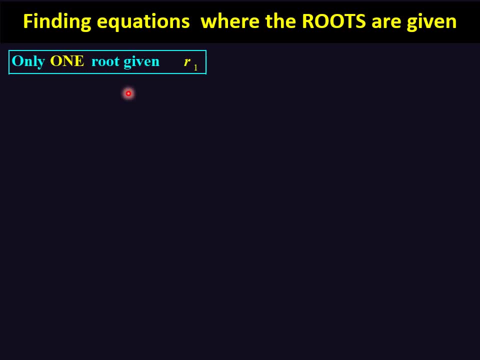 Let's look at the following situation. We're only 1. Real root is given. There we have it graphically. What is the real root? R1.. Now we're going to consider the cubic equation in this form: What is the one root? 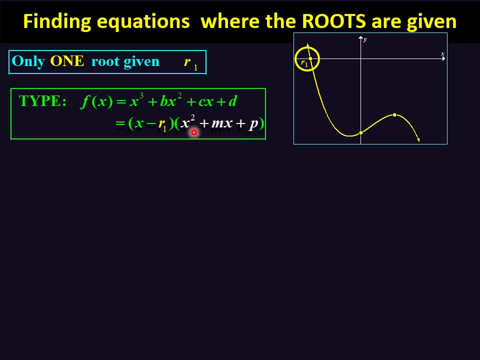 R1.. So we have x minus R1.. And the other factor of the cubic here would be quadratic, Which has non-real root: x squared plus mx plus p. Let's take an example: What is the real root here? x equal to 3.. 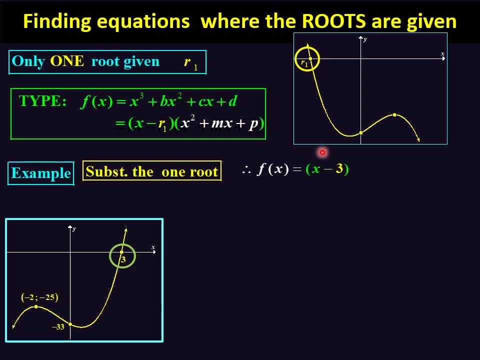 So let's substitute that one root. There's a positive 3. So I end up with x minus 3.. Then we have a quadratic And there is a quadratic x squared plus mx plus p. Because we have two unknowns, m and p. I need two points. 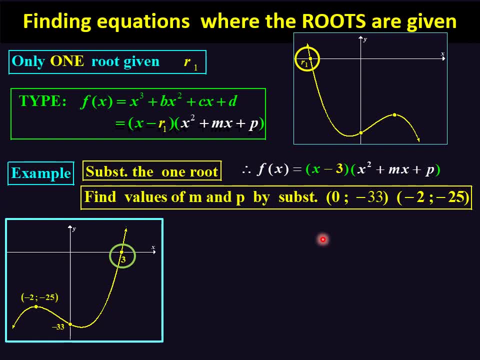 And what are the two points? Let's look for them: 0 and negative 33 and negative 2 and negative 25.. Which one would be the easy one to substitute? That's correct, The 0 and the negative 33.. 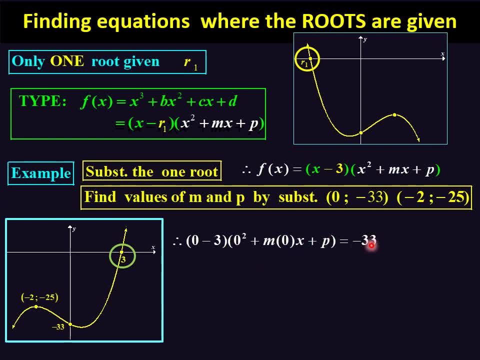 So let's substitute that. There I've inserted 0 and there's my negative 33.. This gives me negative 3, p equal to negative 33, which leads us to p equal to 11.. Now we're going to substitute the negative 2 and the negative 25.. 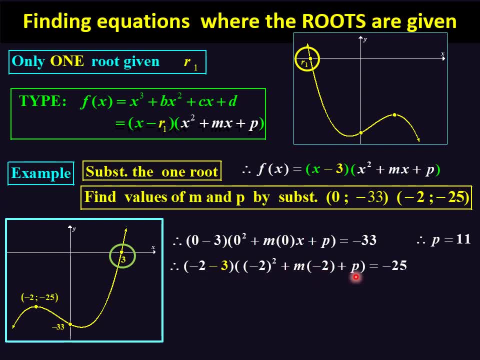 There we substitute the negative 2, negative 2, negative 2.. And remember, This is a 11.. So I end up here with negative 5 p equal to negative 25,, which leaves us with m equal to 5.. 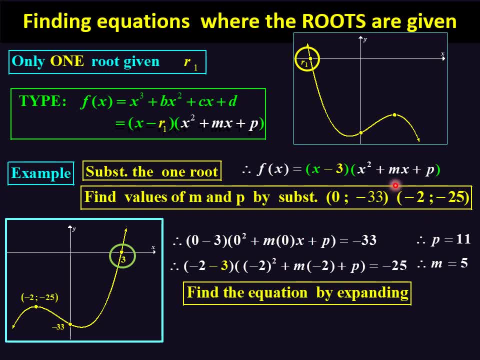 Now I can expand. I now know what the m and the p is, So I insert the m value and the p value And I just expand that And I end up with a cubic expression: x, cubed plus 2x, squared, minus 4x minus 33.. 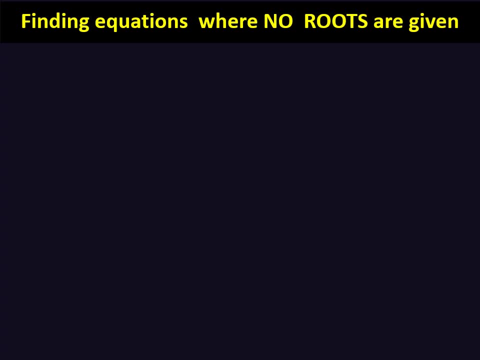 Now let's look at examples here where there are no roots given. We have three points. Let's say you look at an example there, We have three points. So we have a turning point in this case and a y-intercept and another turning. 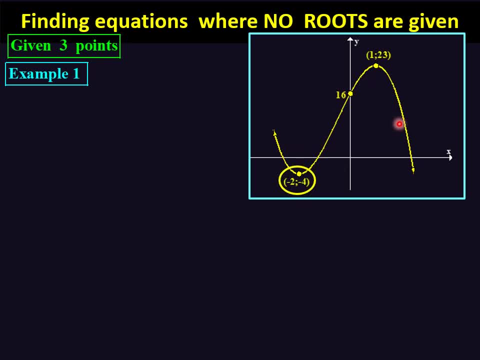 So we've got three sets of points there, But no roots. See, there are no roots. There is a point, There is a point And we also have a y-intercept. Let's look at this: There's a p and a q and a r. 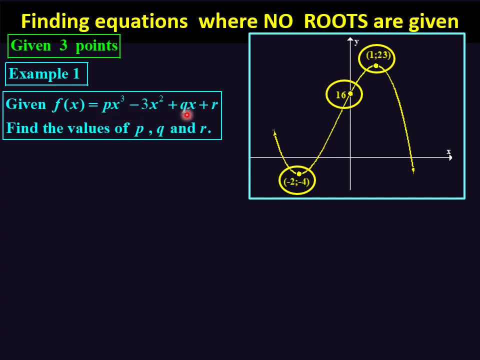 So there are three unknowns. So there's three unknowns. We should have 1,, 2,, 3, right 3 would be sufficient to be able to. We need 3.. So again there we start with the easier one, which is 0 and 16.. 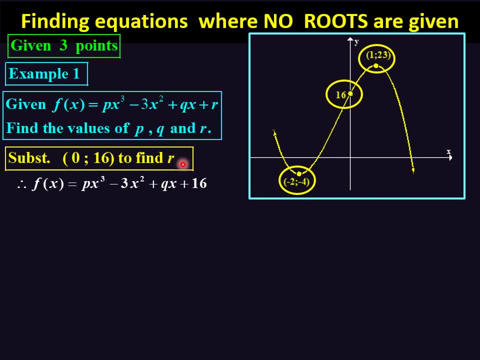 Substitute 0 and 16. So the r becomes a 16. So r is already equal to 16.. Now we need to find the p and the q. To do that, we substitute 1 and 23. And negative 2 and negative 4.. 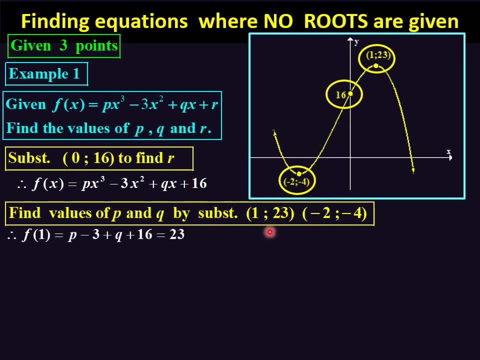 Maybe it's easier to start with a positive. Let's substitute. Let's substitute the positive value in first, And then we end up with a linear p plus q equal to 10.. Now let's take the negative. Let's be more careful with the negative. 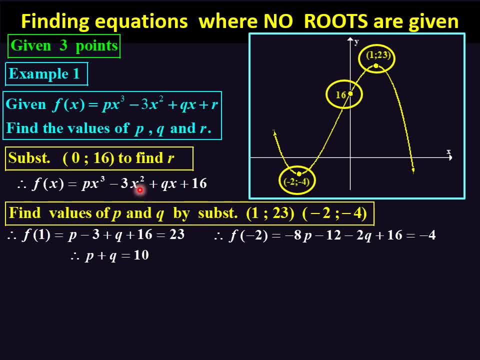 Negative 2 cubed is negative 8. That's going to be 4 times negative 3,, which is 12. That's negative 2 cubed plus 16. And if we simplify that we end up with 4p plus q. 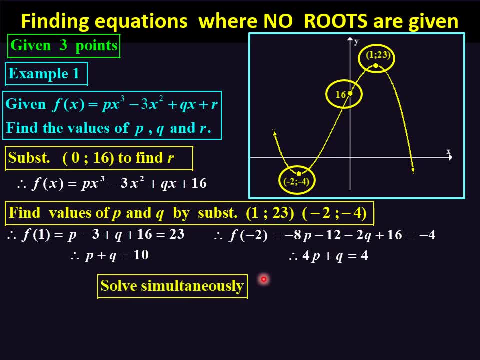 So now we have to solve simultaneously. Now remember, you can either do it by elimination or substitution, or use your calculator. Whichever method you used, the correct value then would be p equal to negative 2 and q equal to 12.. 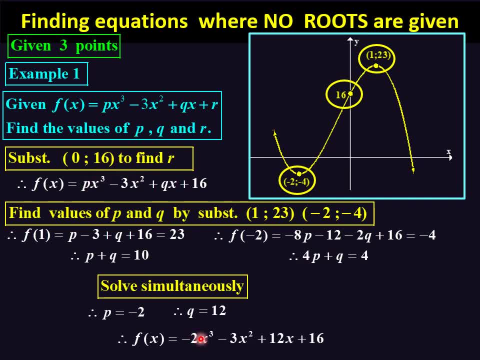 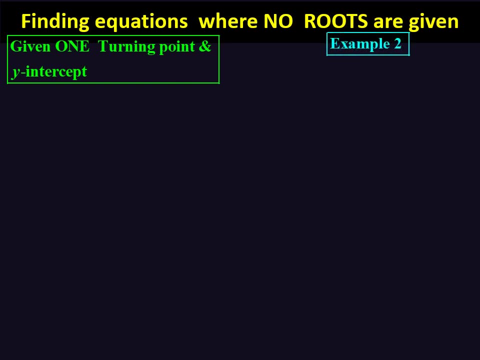 Then we substitute the p, and we substitute the q, And we've already worked out the 16.. And there's my cubic equation Example. This one is slightly different. We don't have two turning points, but one turning point. Okay, 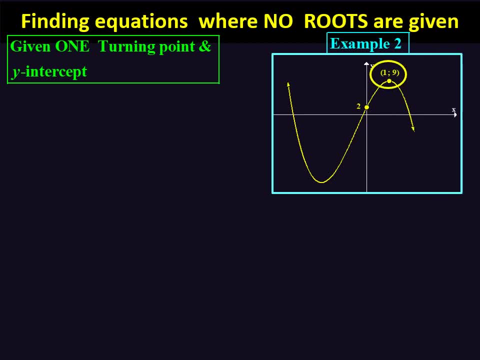 How do we find the cubic equation if you only have one turning point? Let's see what we have there. There we have the form of the equation: How many missing values there? a, b and c? So that means I need three points. 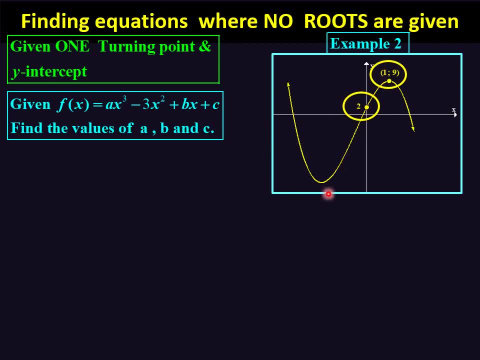 When I look there, there's no other point. You know there's nothing hidden there. There's a 2 and a 1 and a 9.. But this is a turning point. I will come back to that turning point Again. start with the easy. 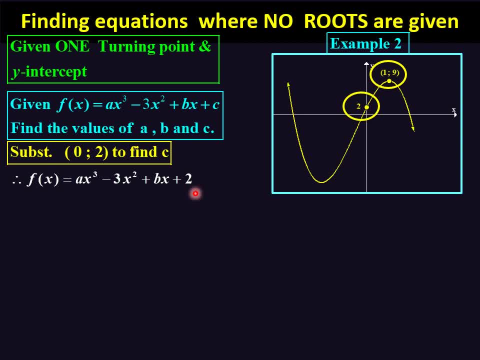 The easier point will be 0 and 2.. That will give you a- c. Now we have two unknowns, So let's substitute the x and the y, In this case 1 and 9.. We substitute that, We end up with a plus b, equal to 10.. 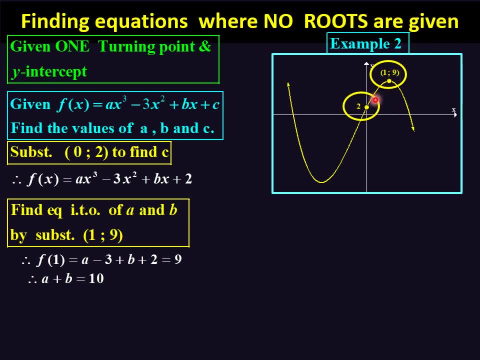 Now we already substituted 1 and 9 and 0 and 2.. There's no other point. What do we do now? But let's see, They mentioned that 1, 9 is a turning point. What do we know about turning points? 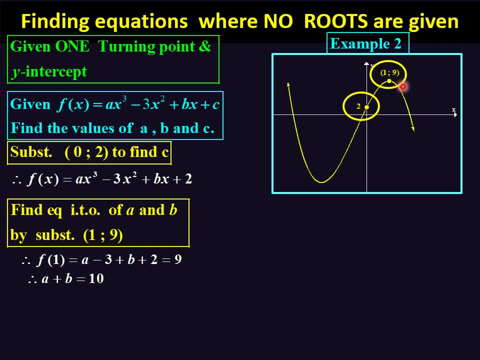 That's correct. The first derivative is equal to 0.. So here we're going to use calculus to assist us further. So we find the first derivative equated to 0.. And x equal to 1 is where the first derivative is 0.. 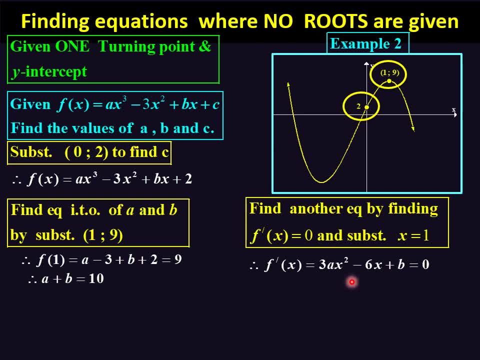 So differentiate. that Gives us 3ax squared minus 6x plus b, equal to 0.. Substitute 1. 1 squared is 1. So that becomes 3a negative 6 plus b, And we can simplify that And that leaves us with 3a plus b equal to 6.. 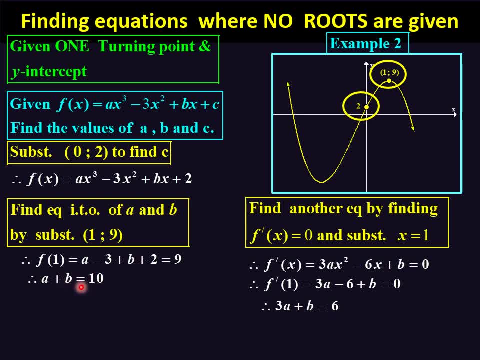 Again two unknowns. So I need two equations. Solve them simultaneously, Whichever technique. What other techniques again? Either substitution or elimination, or just use your calculator. a equal to negative 2. And b equal to 12 are the two values. 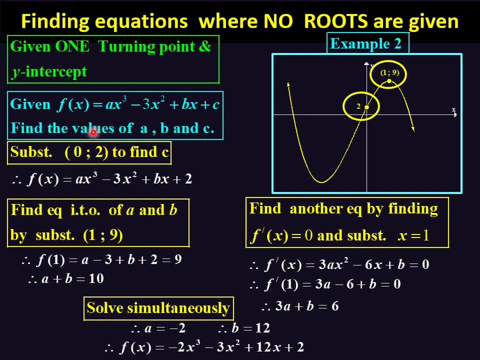 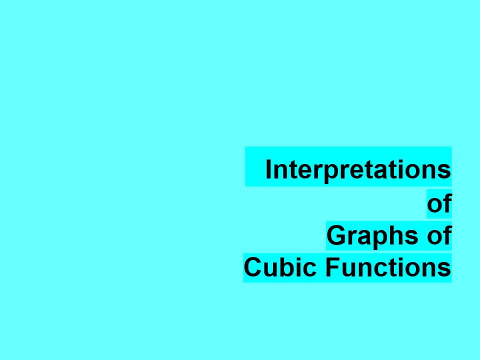 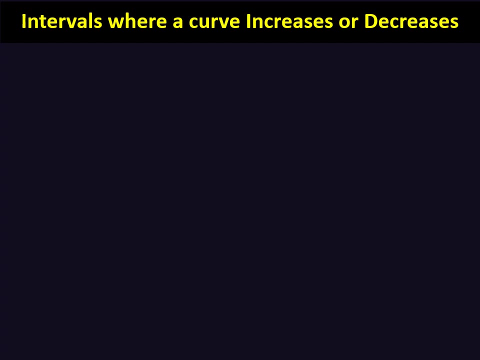 And once you have the values, you can write down the equation there. Now, next, we're going to look at interpretation of graphs of cubic functions and, specifically, some inequality relationships we're going to look at. Okay, Let's look at where a curve increases or decreases. 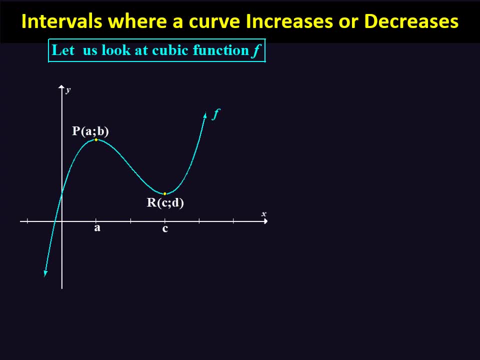 Let's look at the cubic function. There we've got a cubic function, And what is this? This point represents here- That's right- The local maximum And this one Local minimum. And at the local minimum I have a value, a associated with it, which is the x coordinate. 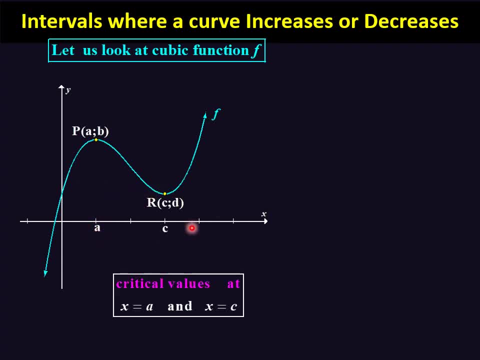 What do we refer to? the a and the c here? That's correct. The critical values, right? Critical values are the x coordinates of the local maximum and the local minimum. Now if I want to find out where the curve increases or decreases, 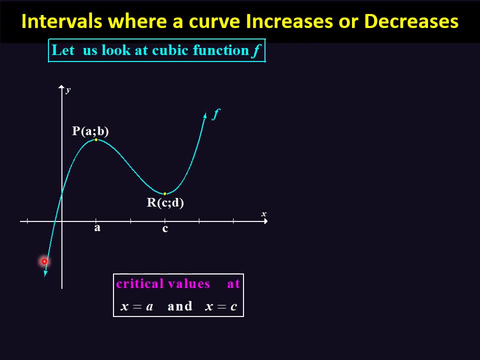 always start from the left side, follow it here. What is happening here? It is increasing, And from there it decrease until it reached the minimum, and then it increase. So the critical values will assist you in determining where a curve increases or decreases. 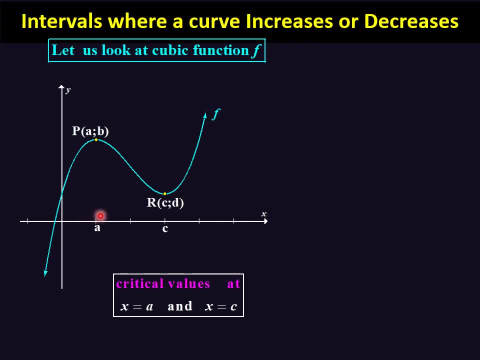 So it increases from this side up to the a, then it decreases again up to the c and then it increases again. so let's do that: increasing. where is it increasing? from negative infinity to a. and increasing means, I mean there is the first derivative- greater than zero. 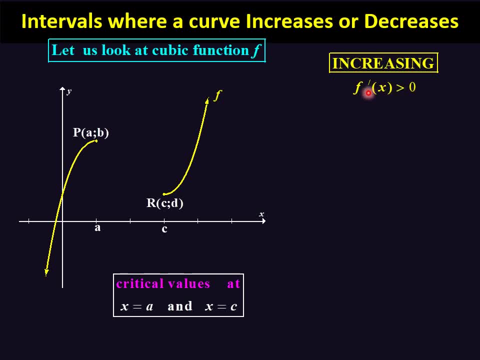 or the gradient is greater than zero, or the m value is greater than zero. so there it's, from negative infinity to a, and then this one is from c to infinity. it's advisable to write it rather in interval notation. it's much simpler to write the intervals where it increases and 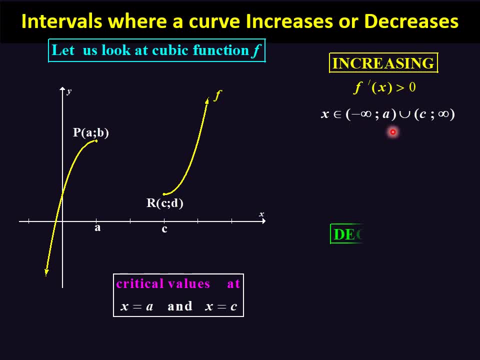 decreases, preferably in interval notation there Decreasing: where did we say it was decreasing? let's see where is it decreasing. it decreases if the gradient is less than zero. and if you now look at the decreasing portion, there's the decreasing, the one in green. I've color-coded the increasing. 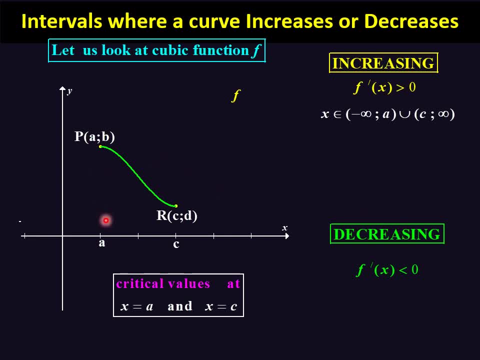 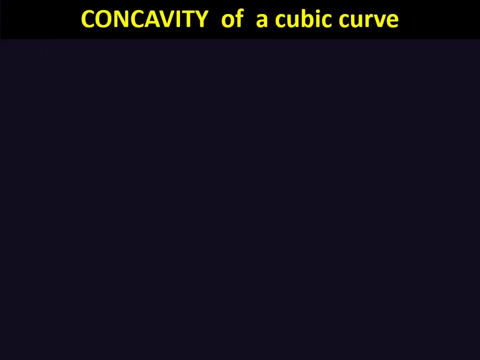 and decreasing is in green and it decreases from A to C between the two critical values. so if we want to determine intervals for increasing and decreasing, we use the turning points. I determine the critical values using the turning points. now, this is another concept we're going to refer to and this is the 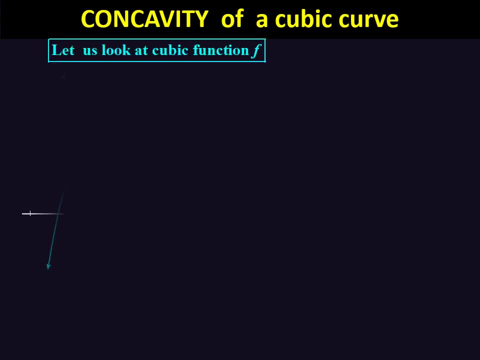 concept of concavity. let's look at our cubic function. there we've got a cubic function and this point here. remember when we sketch curve, what was? what was this one? that's right, this is the local maximum and this one is the local minimum. but what is this one here? this is the inflection point. you still 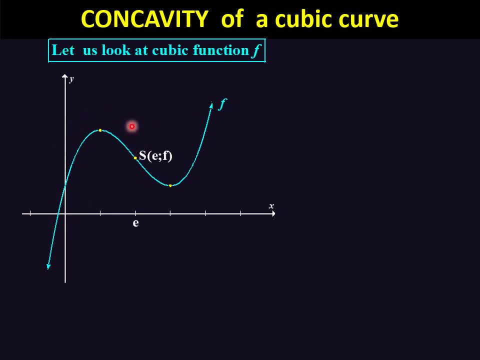 remember- there is a point here, and there is a point here, and there is a point here- the tangent was above the curve and at the inflection the tangent is, it will then be below the curve there again. in this situation and here we have a critical value associated with that inflection and that's the X coordinate. 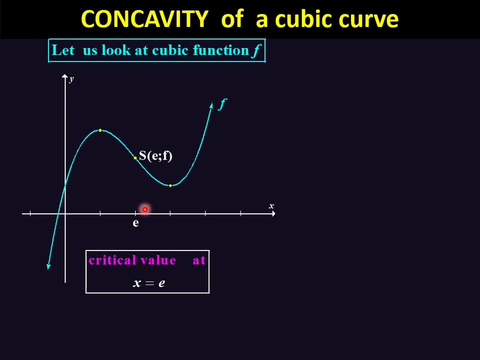 of the critical value. how do we determine critical value of inflection? that's correct. we find the second derivative. so let's just see. look at this graph now. so if I look on the left side of my inflection point, this part of the curve right, can you see there's the inflection, and I go to the turning and I 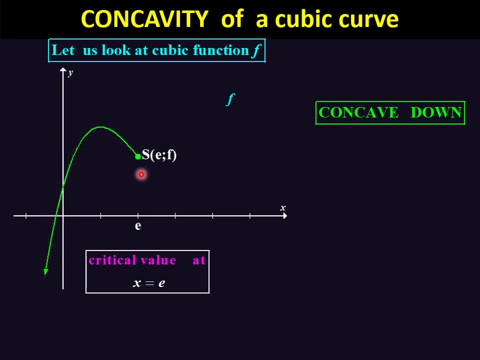 turn and it just goes down, down, down, down. right. this type of curvature is known as concave, concave down, and actually the arrow can help you also to determine that. see there, it goes down. that way that's concave down. so on the left side of the curve it's going down, and it's going down, and it's going down. 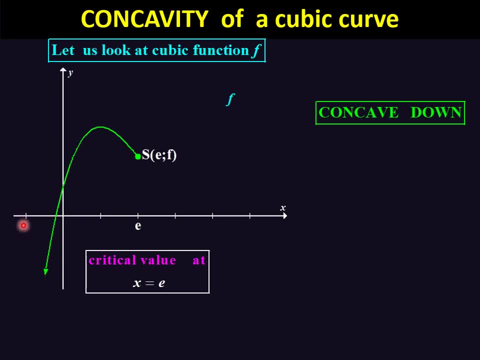 left of the inflection point and on the left there would be: what will the interval be? that's correct, from negative infinity to e. so the second derivative must be negative. then x will be between negative infinity and the critical value of the inflection point there right. let's look at the other one. 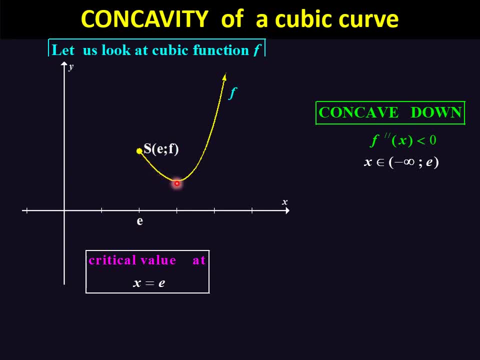 now you can even see there. it's from the inflection. it turned and it went up. so this type of curvature here is known as concave of let the arrow sort of assist you in determine the type of concavity. and you can see it's from the inflection point on the right side of the inflection point. 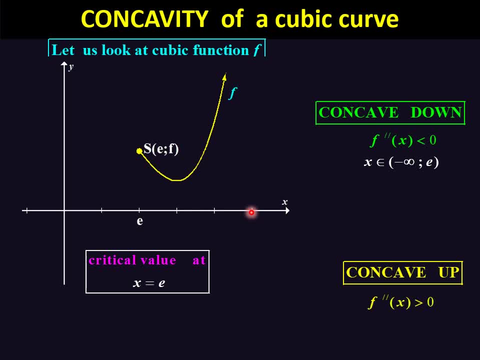 so that is concave up and concave up when the second derivative is greater than zero. in this case it's from on the right side of the inflection point, that is, from e to infinity right. and you just look at the two graphs there you can see the concave up. concave down is the one in green. 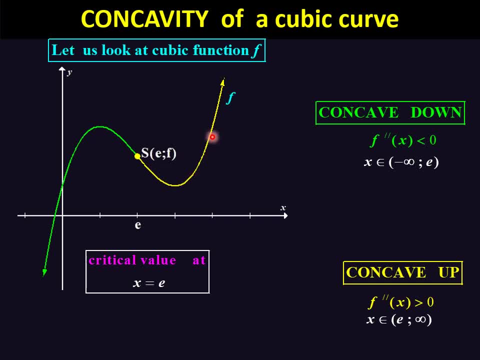 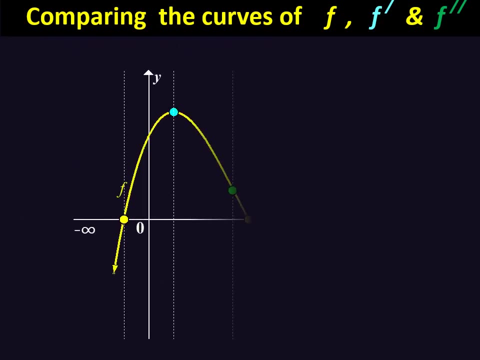 and concave up is the one, and let it from the inflection. you can see it goes up that way and the inflection point is where the concavity changes. it changes from up to down. now we want to compare the different curves right, the function, its first derivative and its second. 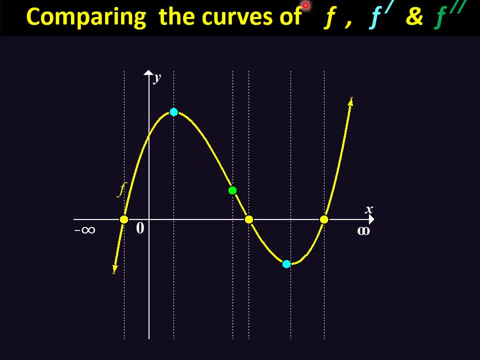 derivative. let's say there's the curve there, so that's the f, that's the one in yellow, that's the. we're going to compare that. and if i look at this curve here, this one has a x-intercept and an x-intercept and an x-intercept, right and there we have. 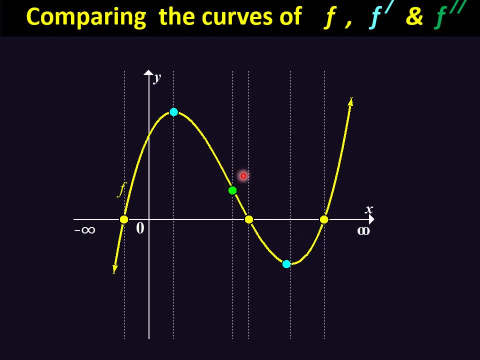 the local maximum and the local minimum, and there we have the inflection point, and now you can see these faint dotted lines there just to help us with the intervals of infinity. to that point, then, from this point up to this one, then from there up to that critical value. 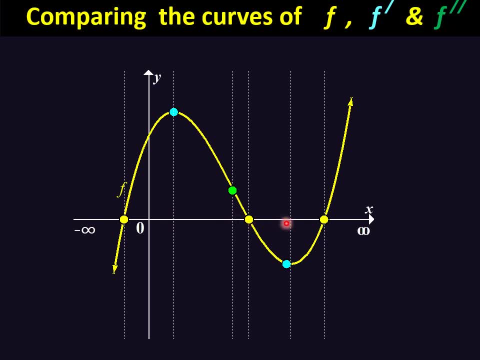 from there to the intercept, then to a critical value, then to an intercept and then to infinity there. So the cubic function is the one there in yellow. When we have the first derivative of a cubic function is a function like this, and which one? which shape? you still recall the shape, that's correct, it's a quadratic. 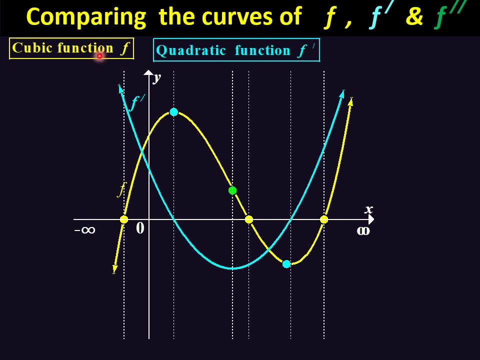 right. so if you have a cubic function, it's first derivative is a quadratic and there's the quadratic there and this quadratic- if you look at it carefully- that critical value for it's local maximum. it becomes the x intercept there right and the critical value for the minimum. 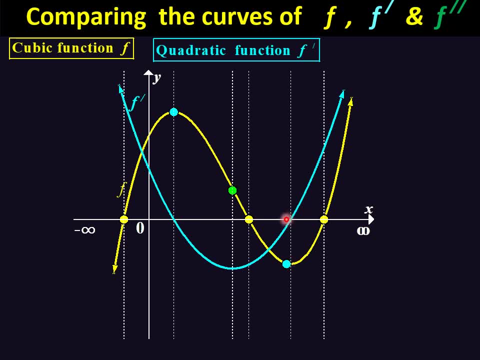 becomes the x intercept of the first derivative. and if you find the second derivative, the second derivative of a cubic is a. that's right, it's a linear function, okay, so this is important for you to know: a cubic function, it's first derivative. 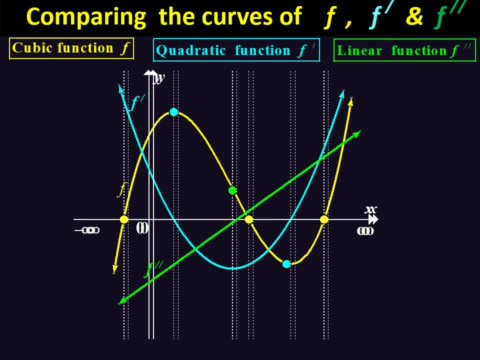 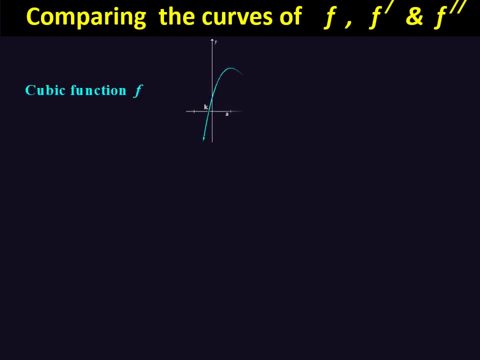 is quadratic and it's second derivative is a linear function. there, Let's just do them individually. there's the cubic function. okay, just a little bit different there. so I have a cubic function here. and what are the x intercepts here? there, the x intercept is at the point k. 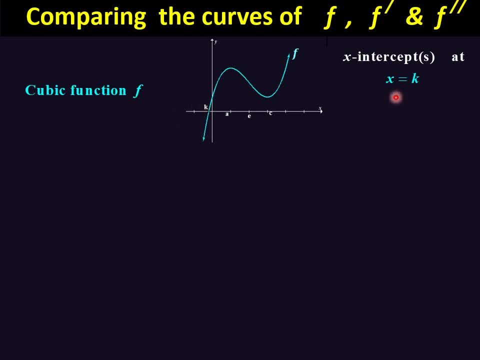 it's a bit small there. there's the x intercept at point k that only has one x intercept. let's look at that same one and let's look at the quadratic function, for that the quadratic is the first derivative. there's it there, right, and you can see the critical value. 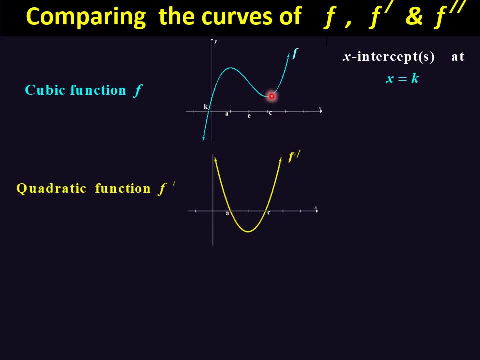 a will match with that x intercept, there the critical value of c for the minimum. so there I have the critical value. so actually the x intercepts of the first derivative and a. the second derivative, is a linear function, and there we have the linear function. 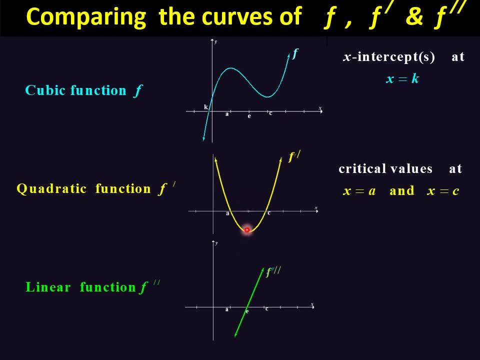 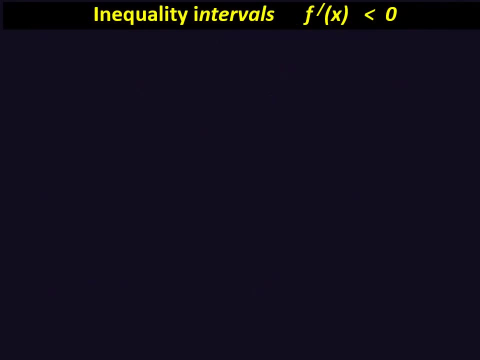 right. and this x intercept corresponds actually with the turning point of the quadratic and that critical value here, that's actually the critical value associated with the inflection point. now let's look at some inequalities. now the inequality interval, for what does this mean? this means the first derivative less than zero. 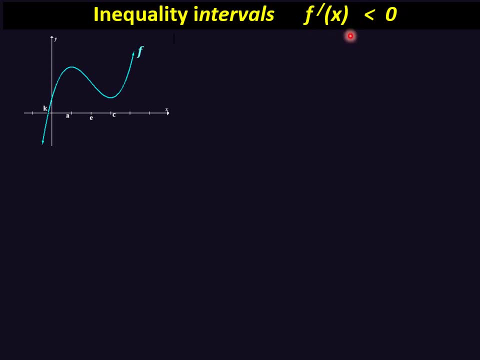 what does first derivative also mean? the gradient is less than zero. if the gradient is less than zero, what does that mean? that's correct. it means the graph is decreasing right? so if I have a first derivative, I look at the critical values and the critical. 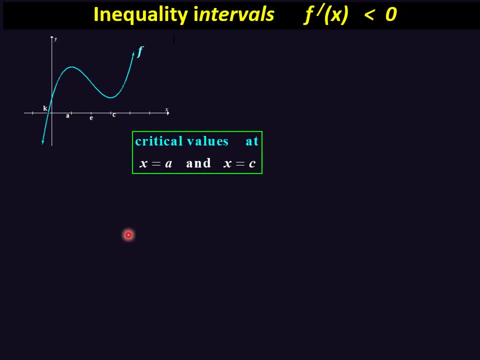 values we obtain from the turning point. so what's there? the critical values are a and c. so that means where's the graph decreasing? can you see where the graph is decreasing? let's follow there. there the graph is increasing and then it decreases. so where does it decrease? that's correct between the two critical. 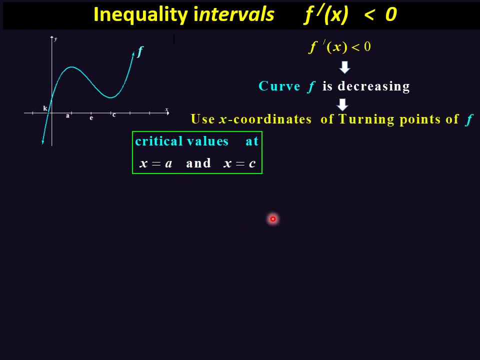 values, so it decreases. there I have to look at the turning point which gives and then it decreases between a and c. let's also look at the second. you see there, this is the original function f and this is its derivative. remember, this is cubic and this becomes quadratic. 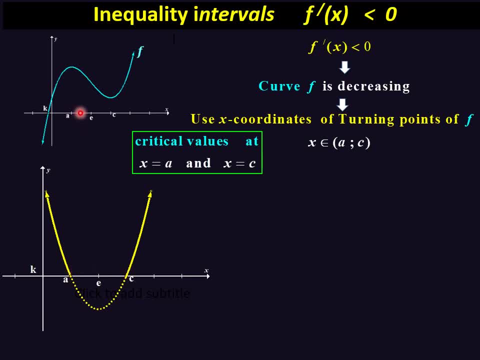 so the x intercepts correspond with the critical values associated with the local maximum and local minimum. so the x intercepts here are actually the same as the critical values for the local maximum and local minimum. so if we have the first derivative, less so I just look at the first derivative. 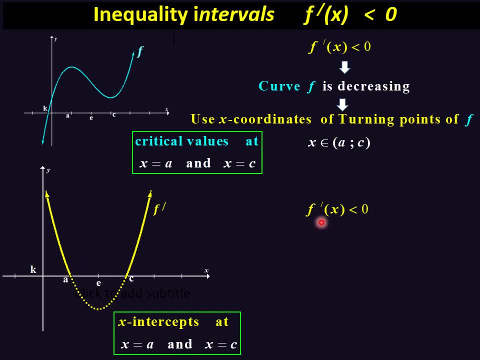 graph, not that one. so where is the first derivative? less than zero? you can see this dotted. there is the less than portion, the solid one is the greater part. so where is it less than that's correct between a and c? so in this case, 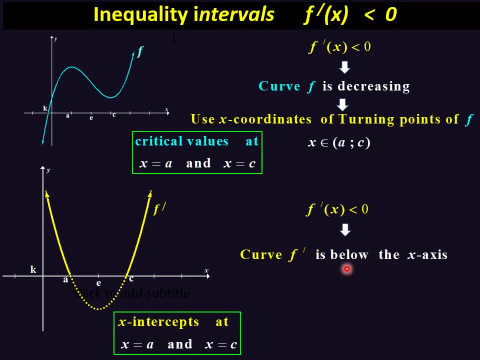 I look at the graph and I look at the portion that is below the x axis. so there I use the x intercepts and it lies between them from a to c, and you see it's exactly the same answer. so if I can find the first derivative, less than, or by looking at the original graph, 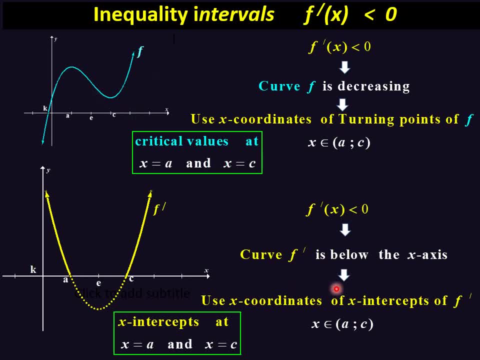 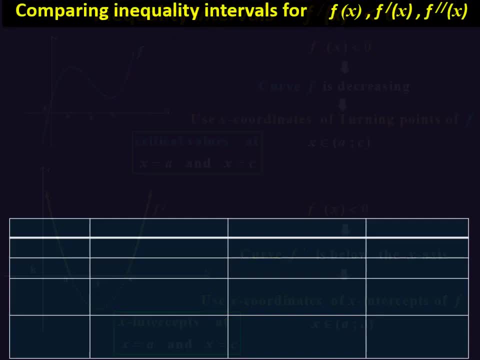 but then I have to look at the critical values there. but if I have the graph of the first derivative, I look at the x intercepts. now, here we're just going to have a summary of a comparison between the intervals for fx and f, prime x and 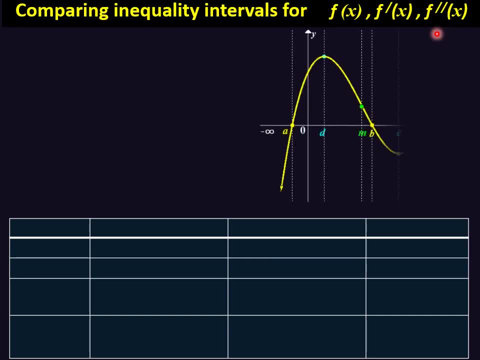 the second derivative there as well. so let's start off with the original function. right, and I've indicated all those various intervals. let's just check again which one is: the d- d associated with the local maximum, and the m, that's right, the m. 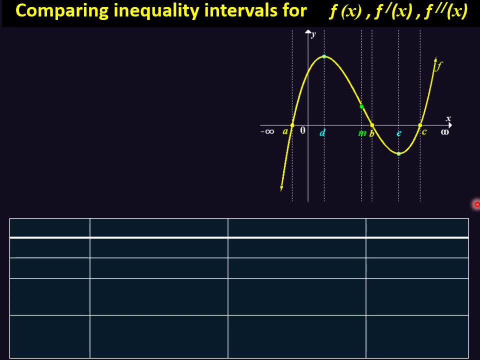 is associated with the inflection point. and let's look at c. c is the x intercept. so let's look at fx now. fx. I'm looking now at the yellow right. we're going to use fx now, and what are the critical values? if I look at my graph there here? 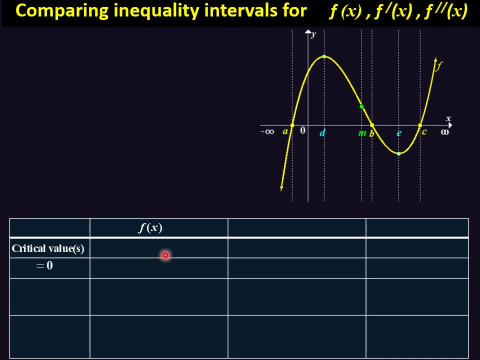 what's going to be critical here would be the if fx is equal to zero, where's fx equal to zero? by looking at the x intercepts. okay, and what are the x intercepts there? in this case it is. let's just look at it. there you can see there's the x intercepts. the x intercepts are. 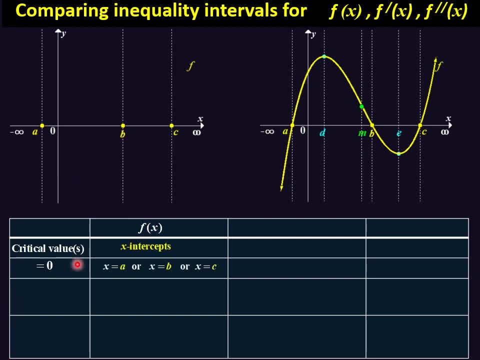 at a, b and c and because I have an equal, my answer is x equal to a, x equal to b and x equal to c. now we want to see where's fx greater than zero fx. so I look at my f graph: where's it greater? 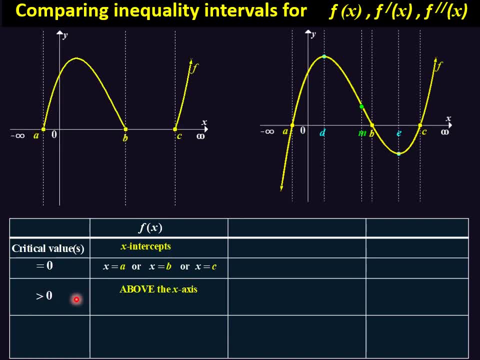 what does greater mean? that's correct. greater means where's it above the x axis. so I look at where's the graph. you see this portion. there's the graph. this is the above portion of the graph and where's it above? that's correct. you have to use your intercept. it's between: 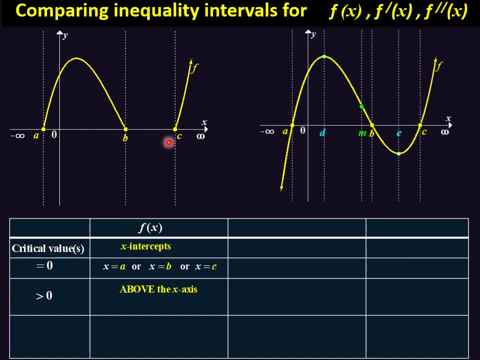 the intercepts there between a and b, and where's it? also, there's another piece that's above, between c and infinity. okay, let's look at where is it. where's the fx below? so I have to look at the below portion. now let's look at the below. 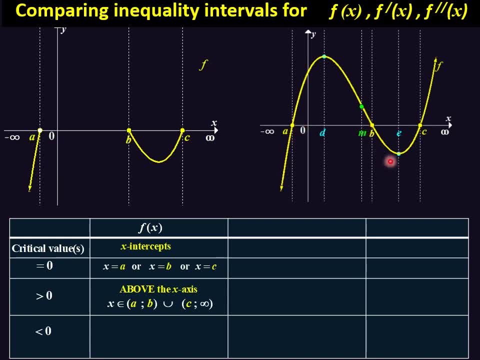 there's the below part. can you see this piece? and this piece is below, so I only focus on the below. you can actually cover up the top part, but if you take a piece of paper, just cover up the top and you. 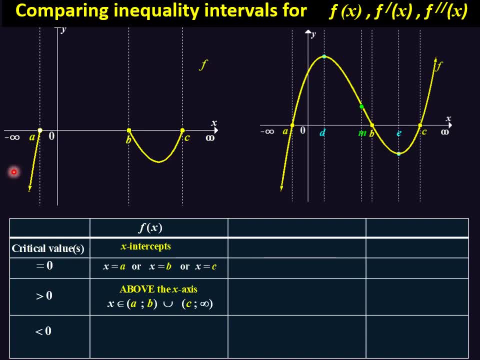 can see where's the less than. and here you see there are two less than portions from negative infinity. so less than naught actually mean below the x axis. so it's between, come again, between negative infinity and a, and then from b to c. 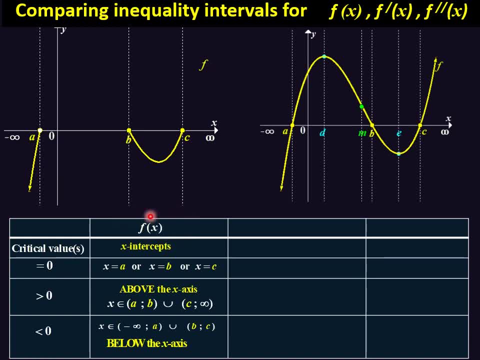 so if you want to find the inequality with fx, use the x intercepts. now we're going to look at- let's take that graph away- we're going to look at the first derivative right now. first derivative means we have to look at what. 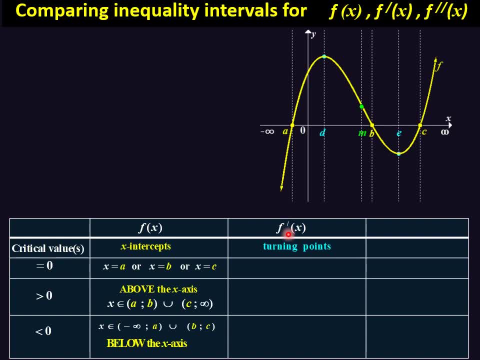 we have to look, that's correct. we have to look at the turning points, right. so the turning points: we've got it here in this nice blue colour and you can see where the turning points occur. the turning points occur- that's correct- at d and there's another one at e, so there, 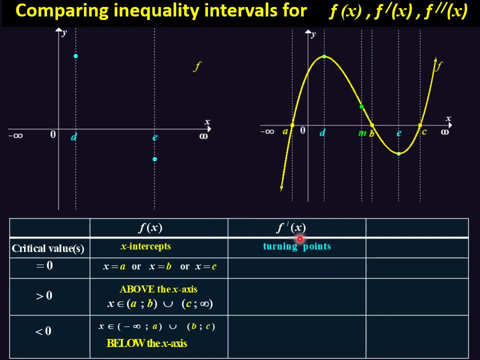 I've got my two turning points. so if you want to do any inequality or any relationship with the first derivative, you need to use your turning points. so I now have the turning points and I now focus on the critical values d and e and the other points. 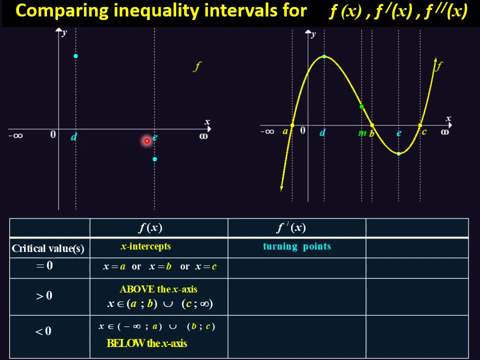 here would be negative infinity and d, and from d to e and from e to infinity. now, where is it that's equal to d and equal to e? but now, if I want to find out where the graph is, let's look at this one. I want to see where is it there's. 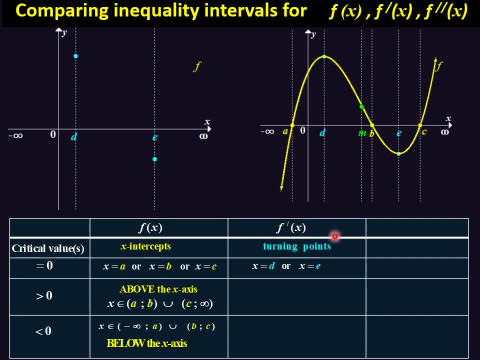 a one greater than zero. what do we mean by first derivative greater come? we had it earlier, that's correct. we have to see. we see there's the greater portion right now. first derivative greater than zero actually means where's the graph increasing? 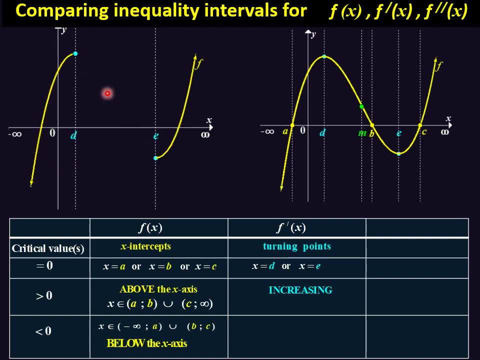 there's the increasing part. it increased. there's the increasing always work from the left side, from increasing there and then increasing there. ok, and you can see it increases from negative infinity to d and from e to infinity. you see, I've used that symbol there. that's a mathematical. 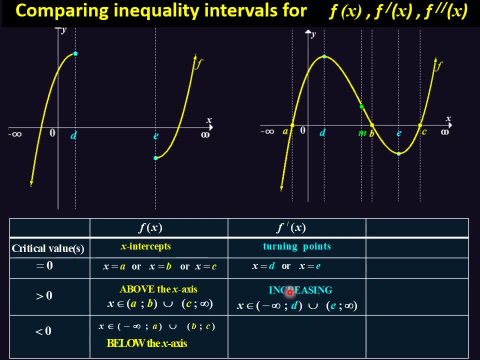 symbol. that means all in mathematics, it's all the same. it's all the same. in mathematics we always try to write symbols, so we're not restricted to a specific language there. we just use that for all right. you can even write in the word: 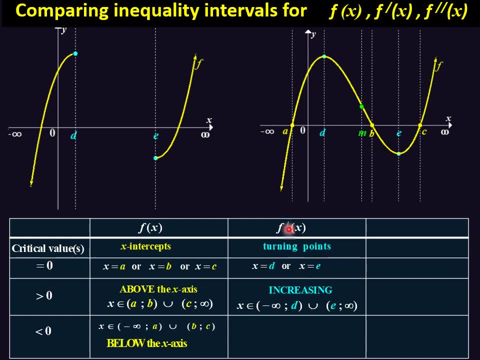 all, it will be acceptable. it is correct anyway. then where's the first derivative: less? if greater was increasing, what would less be? can you picture the decreasing? that's right, just look, let's see. now there's the decreasing. you see, there's decreasing and it decreases. 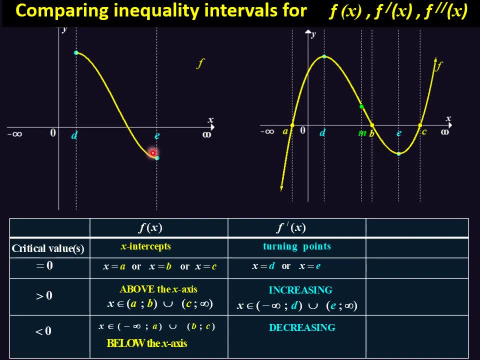 between the two critical values there, from the maximum to the minimum. so decreasing is between d and e. now let's look at the second derivative. let's take that away. let's look at the second derivative. second derivative: the critical values you obtain from your inflection point. 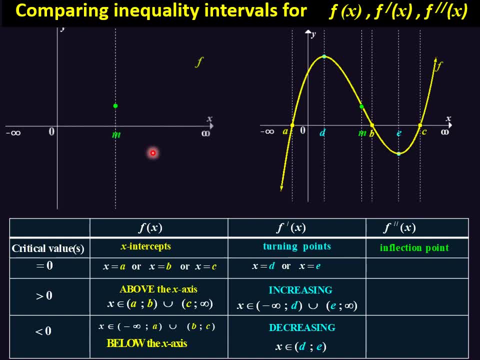 what is the inflection point? there's only one inflection point. let's find the inflection point that's right at m. so we're only going to use this interval: negative infinity to m and m to infinity, nothing else. so when you work, 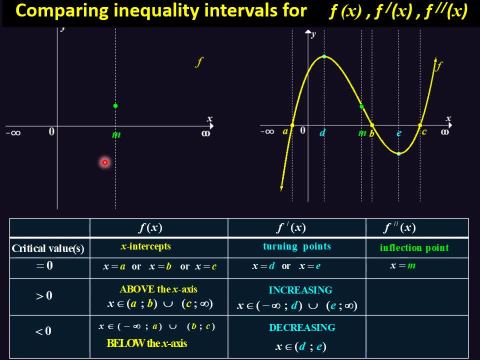 with the second derivative. you only use the inflection point. where's the inflection point? x, equal to m. now let's look at second derivative greater than zero. there it means that's the second derivative greater than zero. and what did we say? that one is just follow it. 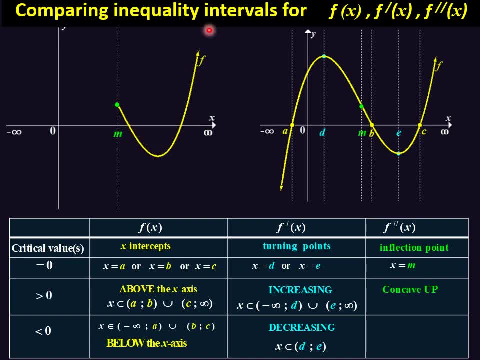 inflection ends going. that's right. we have to look. greater than zero means where is it concave up, and you can see it's concave up on which side of the critical value- in this case on the right side, but always on the right- depends on the shape of the graph. 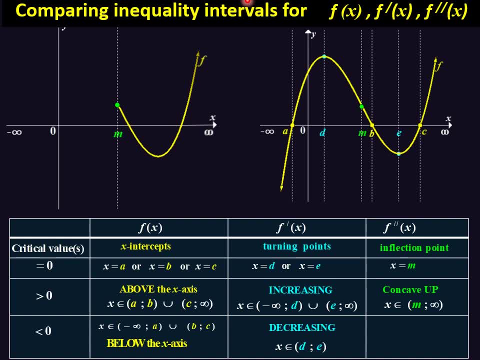 and that's from m to infinity. the less, then means where is it that's right? concave down. see, there's the concave down. inflection: don't look at this, it's not going up. it's going up, but it turns so that. 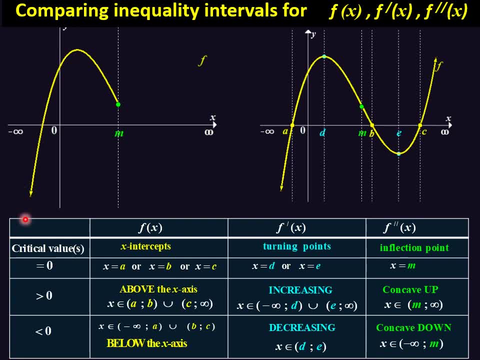 is concave down and it's from negative infinity to m, so that there gives you a nice summary. so when you have the function only you use the x intercepts, when it's the first derivative, you use the turning points, critical values, and when it's the second derivative you focus on the inflection. 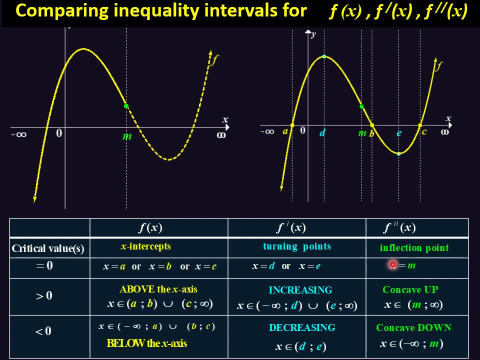 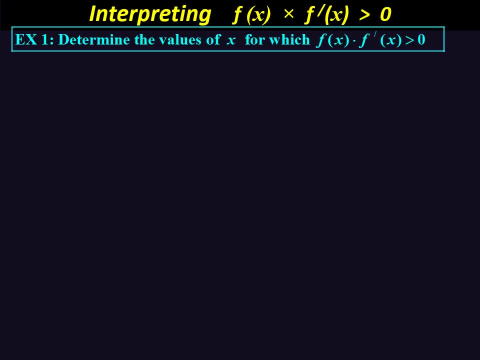 point, and there I'm just putting that back again, right. so there you can see which one this is the down and the other one is the up. now, here we're going to look at one which is actually a level 4 type of question where we're going to 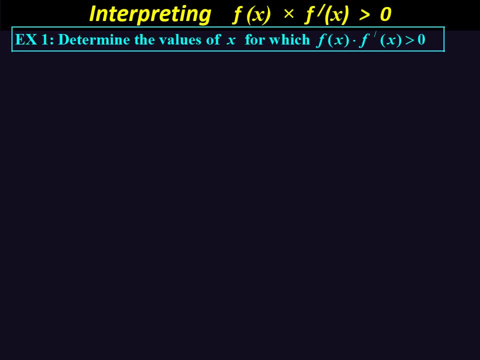 interpret f times it's derivative right or some a few other inequalities that we have here. so let's take our function there again. there's our cubic function there and we've got all the points. you also know what these ones mean. that's the local maximum local. 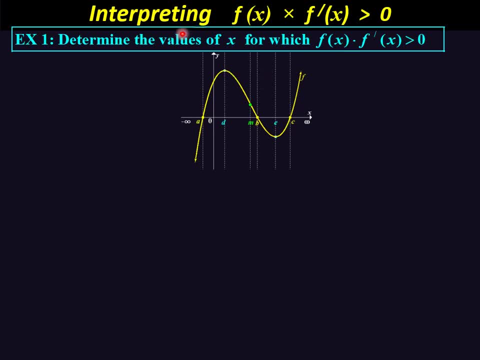 minimum, there's the inflection. those are the x intercepts. you do not use y because we say: determine the values of x. so let's look at this here to be able to understand: greater than zero. what does greater than zero mean? 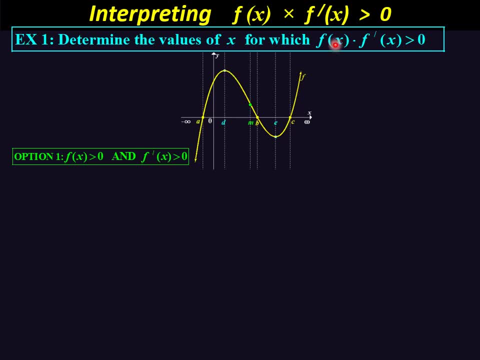 greater than zero means positive. now, what times? what gives you a positive number? come from grade 5 already: positive times positive or negative times negative. so I'm going to look at the two options where the f is positive and the same time, the first derivative must. 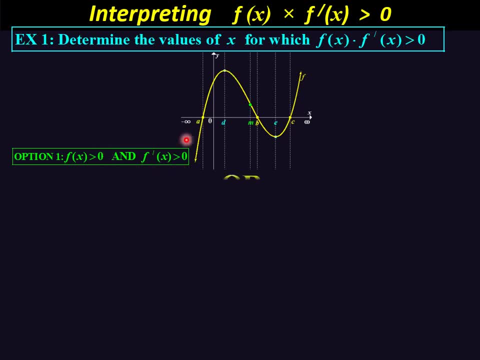 be positive, positive times positive, okay, or we can have the other option: we can have negative times negative. so we're going to look at both. let's look at each one separately: positive times positive, and then negative times negative. now let's look at the. 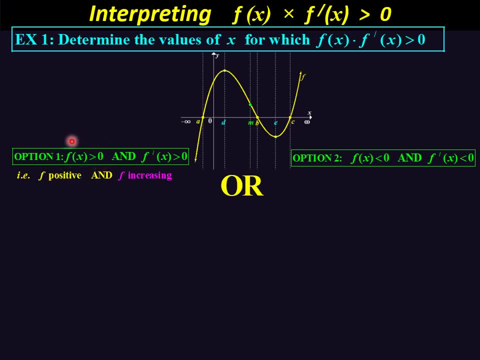 f positive first. so what does this mean? this means the f must be positive. where is the graph positive? and the same time, where is it increasing? so let's look at this. here can you see? there is the positive part of the graph. so first try to see where is it positive. there is it. 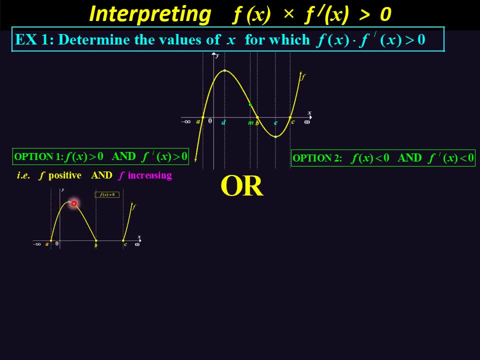 increasing. so there you know, there it is positive. now let's look at this positive part of the graph and which part of it is increasing. what is it doing there? increasing in that part, decreasing in this part, that's correct, increasing. so how many increasing parts do we have, that's? 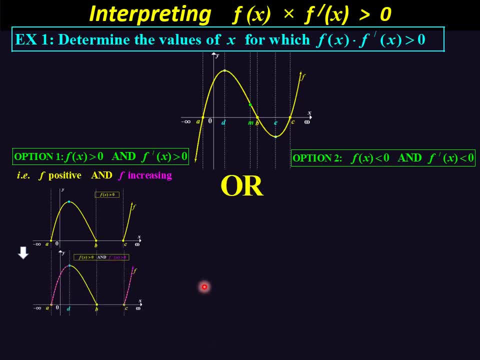 correct, right. so if we look at that and now I've put in shaded in the increasing, there is increasing and there is increasing. now we can write the answer down from you can see it increases from the x intercept to the. 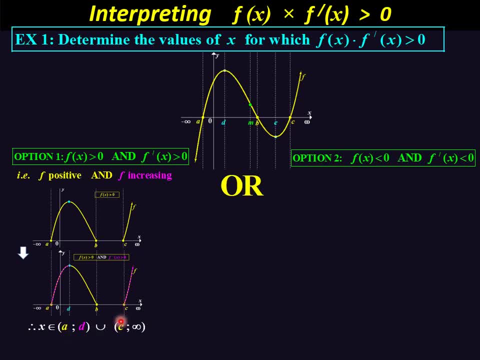 turning point. that's from a to d, then it's from the x intercept, which is c, up to infinity there. so this is the one option that we have. let's look at the other option. when I say that means, where is the graph negative? where does negative mean? 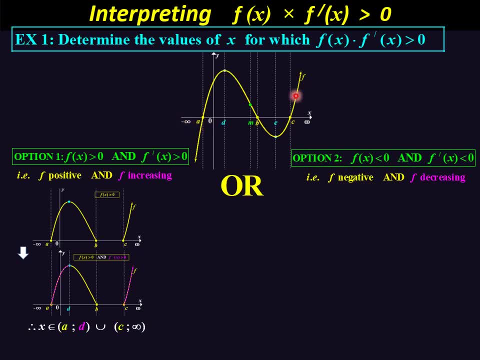 where is the graph below? see what you can do. you can cover up the top and let's look at the bottom part of the graph. there is the bottom part. you see, I only have the bottom part of the function, the portion below. 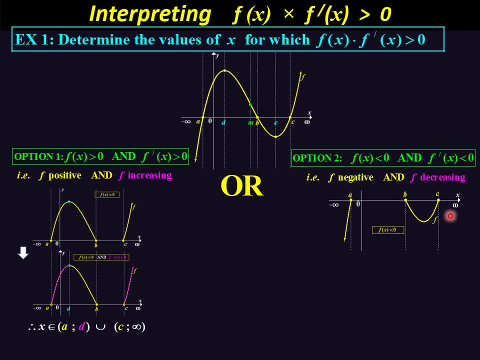 the x axis. now, if we look at the one below, we must now see which part of it decreases. what is this one doing? increasing in this one, decreasing in that one, increasing, so it increases. if you look at that, you see. so the only place where this 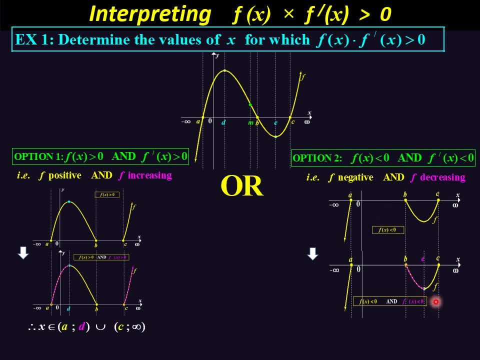 decreases, there is only decreasing portion. so that's from b to e and we can write that down: b to e. now we can just combine them. see, if you write it down like this and you put a o in that, perfect, or you can just write it. 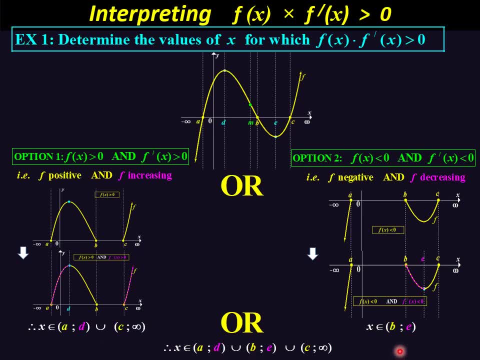 there from a to d or b to e or c. it doesn't matter in which order you put it. I just place it in the order as it appears there, you know, first from a to d, then from b to e and then from c to infinity. but even if 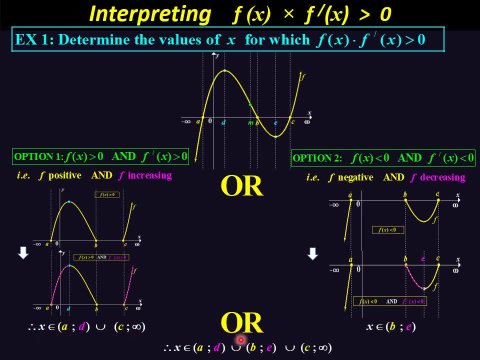 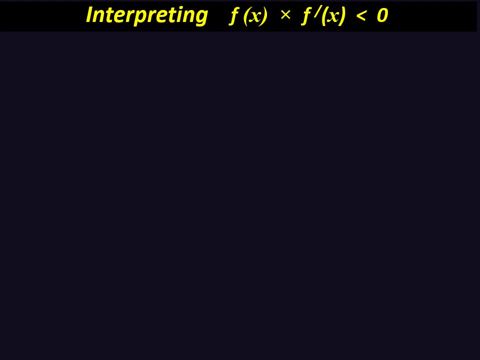 you wrote the answer just like that. it will be acceptable. you can also put the word or in between. so please remember, don't look at the one situation. positive can be positive times positive, or it can be negative times negative. in the previous example we looked at the product. where the product 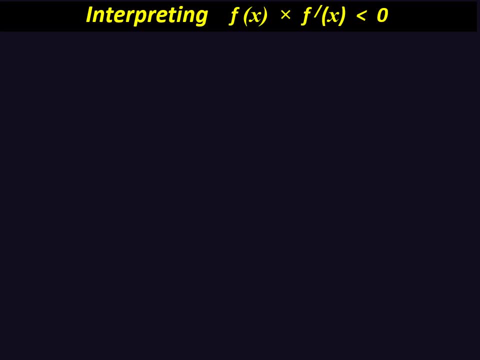 was positive. here we're going to look at where the product is. what does less than zero mean? where the product is negative. now, what times? what gives me a negative? that's correct. a positive times, a negative, or a negative times, a positive, right? let's look at our function again. there we've got the function with all. 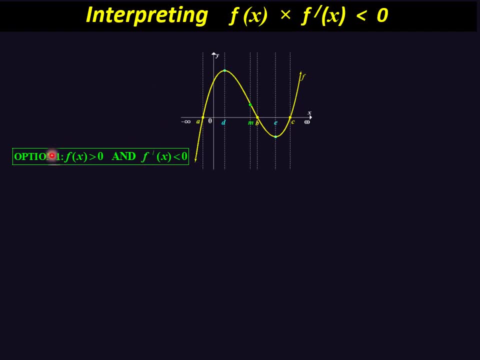 the intercepts and all the critical values. so we're going to look at where the graph is positive. what does positive mean? look at the portion of the graph that's above and then, looking at that above portion, we'll have to check where is it now decreasing? 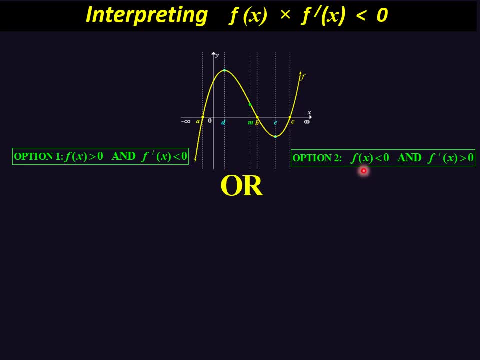 then we have the other option. I can look at below the graph and then, looking at the below graph, below the x-axis, I then have to see where is it increasing. let's do that, this one. you have to be very careful when you do that. 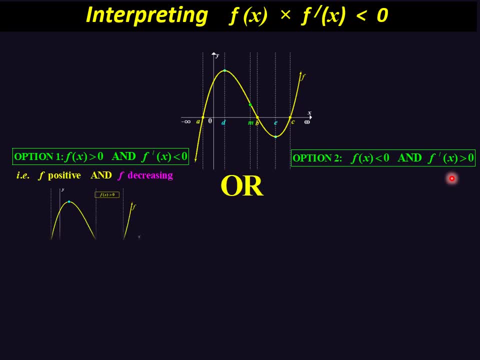 f. positive means above. so let's look at the above portion. there's the above portion. now, of the above portion, which part of it is decreasing? that's increasing. that's decreasing. how many decreasing parts are there? only one right, let's see there. 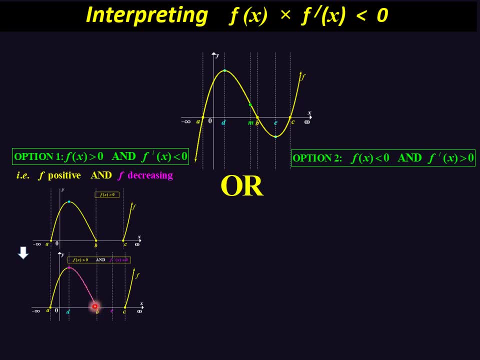 there's it. you see there's the decreasing part there. right, I've color coded there. there's the decreasing and where's the decreasing now from D to B, so I can write down the interval. let's do the other one. you have to look at below the 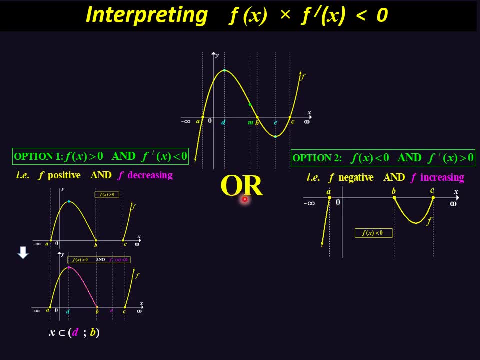 x-axis again. so I look at below, just don't focus on the above, and of the below I must see where is it increasing? there it increases, there it decreases and there it increases there. so let's look at that and there are two parts where it increases. 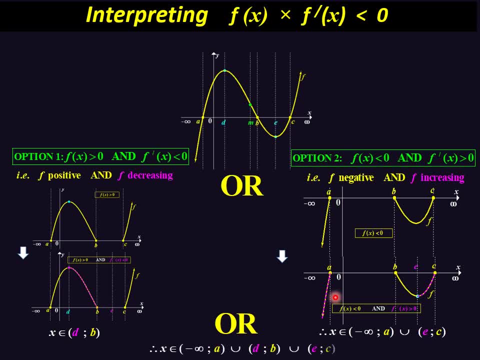 and if I write that down and it's the O, you can just write it like that. but you can just bring them together from D to B. that's in the middle. that negative comes on this side. but if you put it in a different order it would be immaterial, right as long as you. 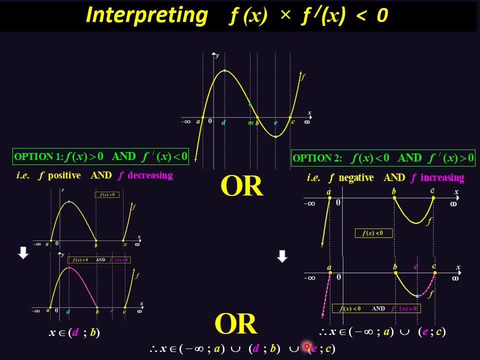 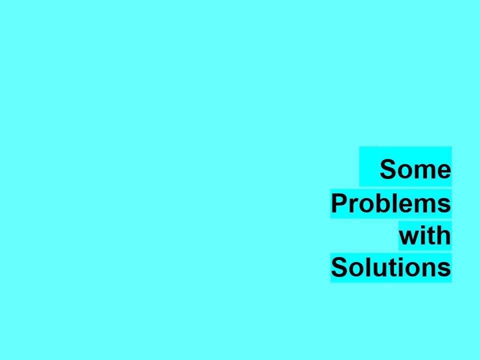 if you're not sure, just leave it like that. you don't have to combine it that way. and that was the question that we look at. the product is 10: 0.. now we're going to look at, actually, some problems that will utilize all these inequalities and interpretations. 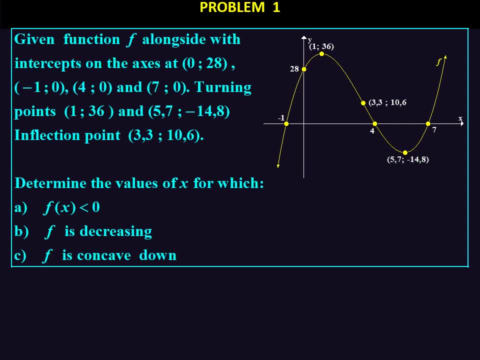 so let's look at the first problem here. let's say we are given a function f, so there's the function f. it's the sketch is given with intercepts and they tell us there's the intercept. just make sure when you read that: negative one and zero, four and zero always. 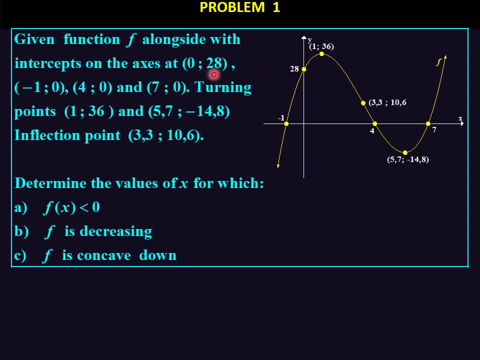 double check whether everything is there. seven and zero, zero. so if it's not there, you insert it. one and thirty six are turned. there's one and thirty six, and normally it's advisable to actually highlight the given information and there's even an inflection point. so maybe this could have been that you had maybe a question. 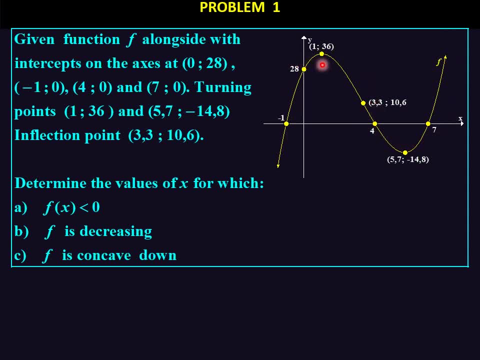 prior to this, you sketch it and all those points were already calculated. then usually a question will. would have now questions based on the graph, right? so you have to read it from the graph. determine the values of x, so the values mean can be more or one. if it's an equal sign will only. 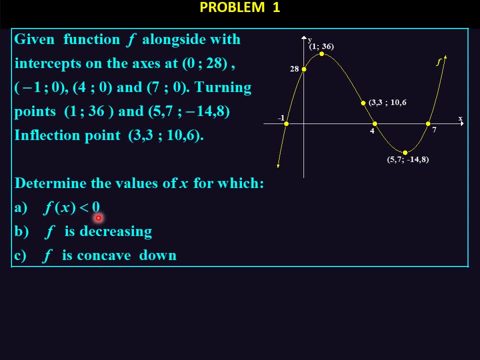 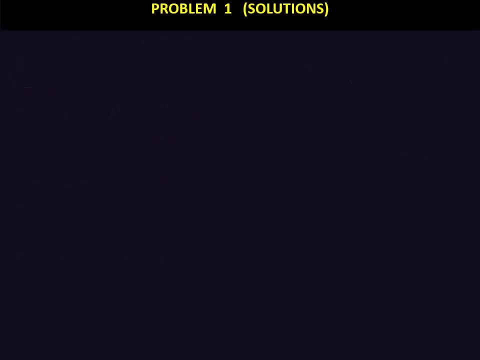 be one right, but if it's an inequality it's normally an interval, so this must be an interval form. interval form. interval form: f less than zero. there we have the given information. let's look at the first question: f less than zero. so which point should we require here? let's correct the x intercepts and what are the x intercepts? 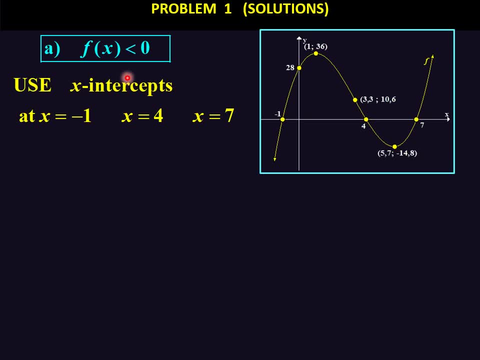 let's look for them: negative one, four and seven. okay, now what does f less than zero mean? how do we interpret that? what must we look for? that's correct. we must look at the value below the x-axis. which part of the function is below the x-axis, which part of the curve is below the x-axis, and can you see the portion below? 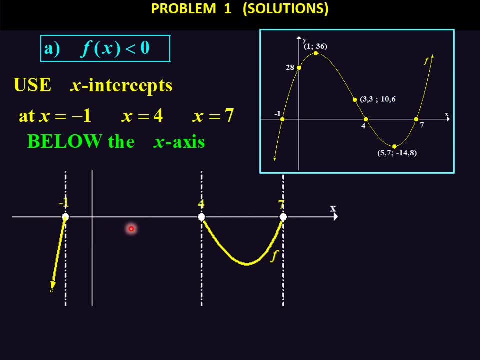 that's correct. there's the portion below, so we just have to write it. now in interval notation we just focus on the x-intercepts, so in this case it is from negative infinity to negative one and the other one is from four to seven. so we've only been using the x-intercepts there. let's look at the second. 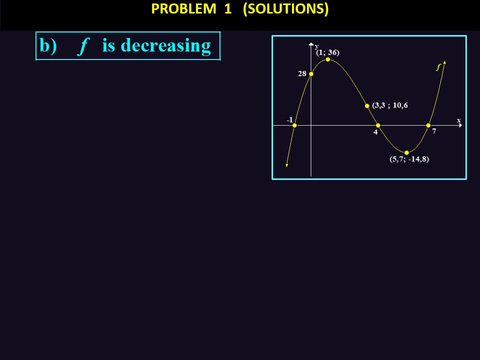 part. let's have the graph back again. f is decreasing. it's quite straightforward. where's the curve decreasing? let's follow this one. what's it doing here? increase and decrease, and in so, which points do we need here for decreasing? that's the turning points. so that is you're going to focus. 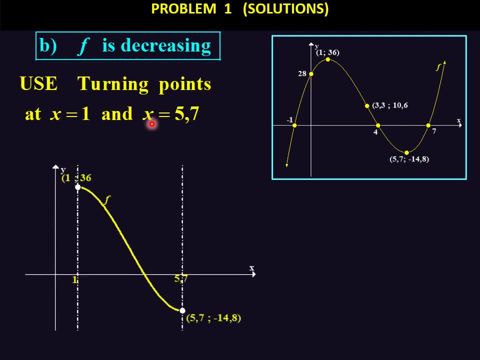 on the turning points, and that's the decreasing portion, as we mentioned earlier. so now we just have to write it in the correct notation: from one to five comma seven. or you could even say x between one and five comma seven, but this one is much simpler and easier to use. i can. 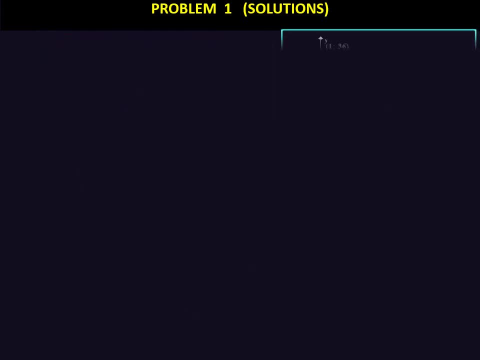 recommend that you use the interpretation. let's look at the third question. f is concave down. so which point do we associate with concavity? that's correct, the inflection point. so where's the inflection point? you see it, that's correct. at x, equal to three comma three. right now, which? 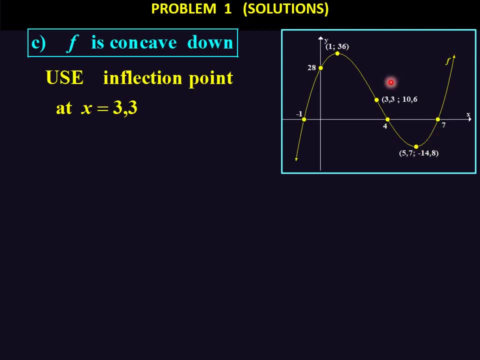 one is this, this one is the. let's follow it. and which one? this one is up and this one is down. so on which side of the inflection point must we must work on the left side. so let's see, there's the inflection point, it goes there, it turns and it goes down. so where's it down on the left side? 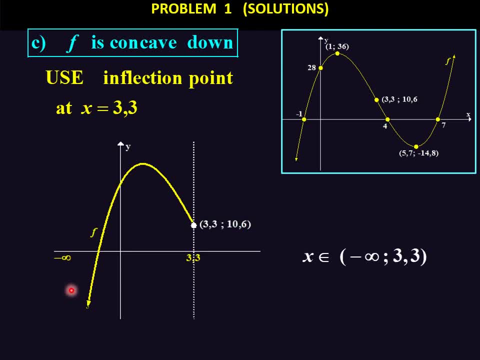 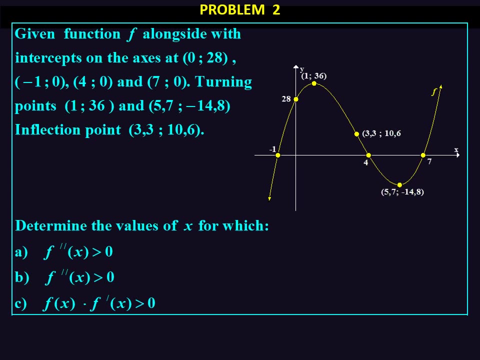 don't write down left side, we just write it in interval notation. if you see, that tells you start there in there. that's easy see where you start and see where you end. let's look at a second example now. there we have the information again. read: see, it's the same graph, but 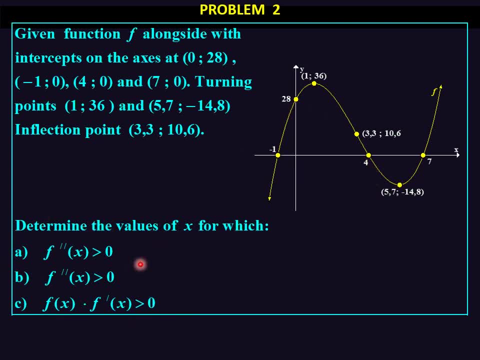 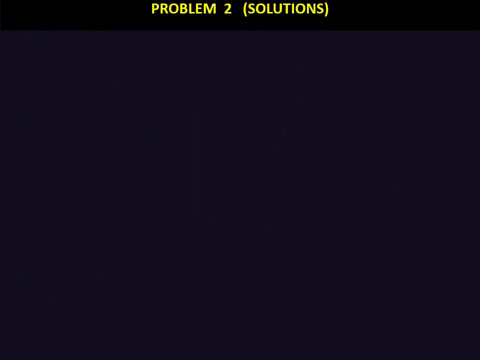 we're just going to have different questions on it. right same points, just different. we're going to see how do we answer the these questions. here there's the graph. let's look at the first one. you see there. there this is a written in function notation: first derivative greater than naught. what does that mean? first derivative greater. 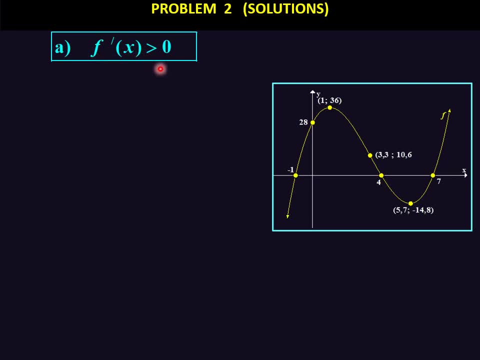 than naught. which points do us we associate with the first derivative that's correct, the turning right. can you see the turning points? and what does first derivative greater than naught also mean? where's the graph increasing? so we need to focus on the turning point, the critical values we get. 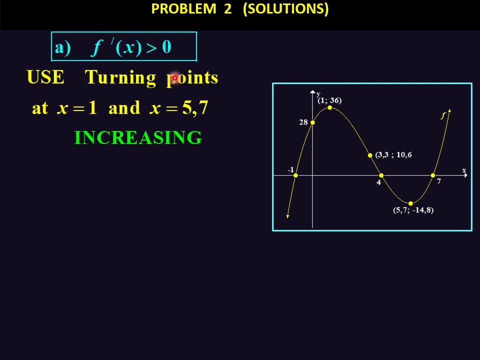 there, and now we're going to see where is it increasing? can you see the increasing portion? let's try to find it. and there's the increasing. can you see that increase? and that increase? that portion that we left out, is the decreasing. now we just have to write that in. see, it's quite easy if you do it this way. work from the left, which. 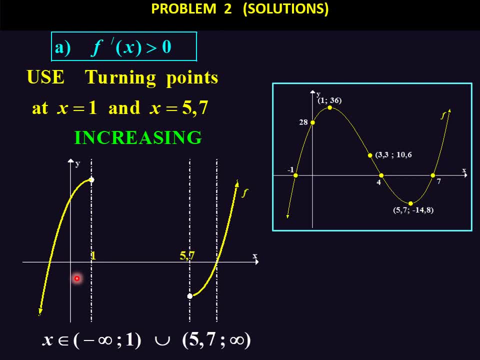 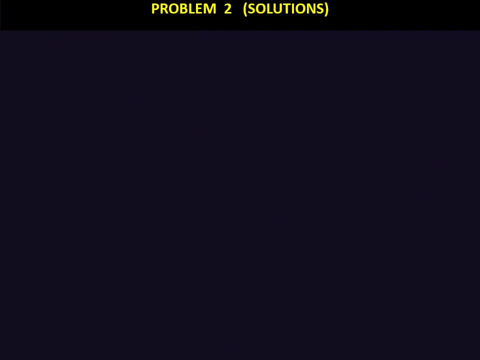 is from negative infinity to one, and then the other portion is five comma seven, seven up to infinity. we always have open intervals here. let's look at the second problem, that's the same graph. what does this mean? see, there's no words here. it's written in mathematical notation. second derivative we associate with: 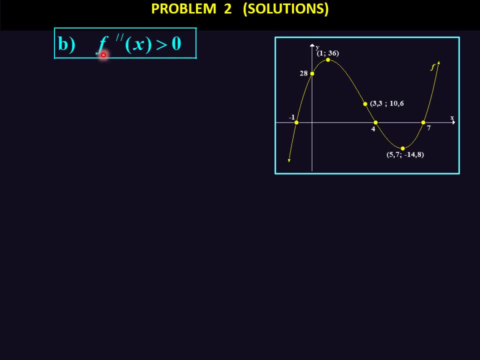 that's correct. the inflection point, and what's the inflection point? critical value: there is x equal to three comma three. right now, what is? second derivative greater than zero mean. that's correct. where's the? the curve, concave, concave up, and you see the up portion. is it the one on the left? 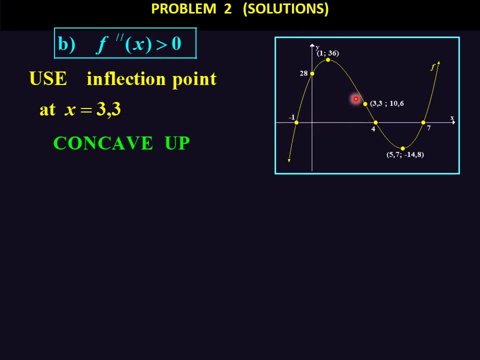 side or on the one on the right side. this one or that one sound like an optician now. so there's the up. you can see there from the inflection turn and it's going up. and this is on the right side. the right side. i need positive infinity. so it's from 3 comma 3 to positive. 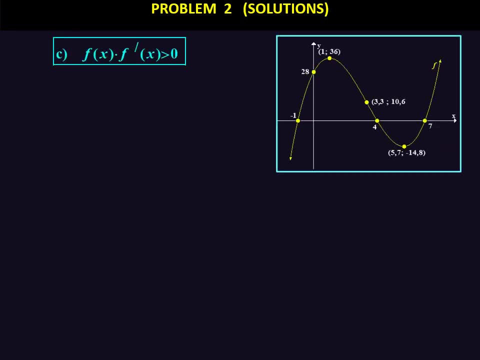 infinite. let's look at the third question. yeah, this is one like we had earlier, and here we have a specific example where we have a product, this product. what does this mean? the product is positive, so we have, we're going for the f, we're going to use the x-intercepts and for the first derivative we're 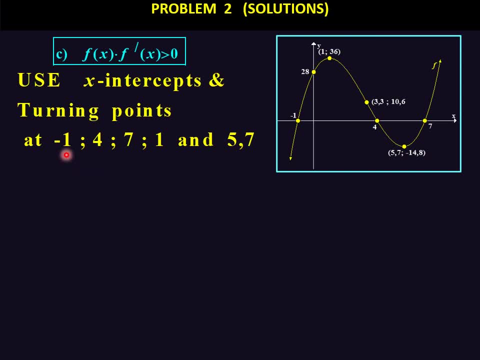 going to focus. so there we have the x-intercepts at negative 1, 4 and 7, and then the turning points are at 1 and 5, comma 7.. but positive, we have two options. so if i say the f graph must be above, 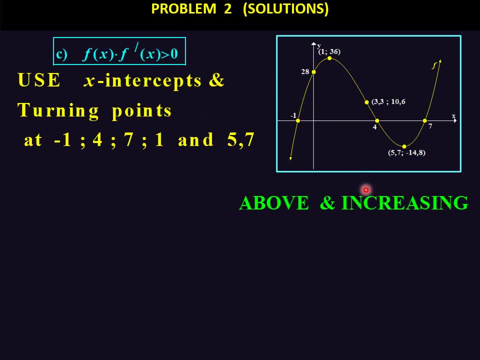 then the same time, i must see where it increases. now look at the other option. opposite of that would be below and decreasing. let's look at, and there we have it. can you see there? this portion is above and it's increasing. this portion is above and it's increasing. 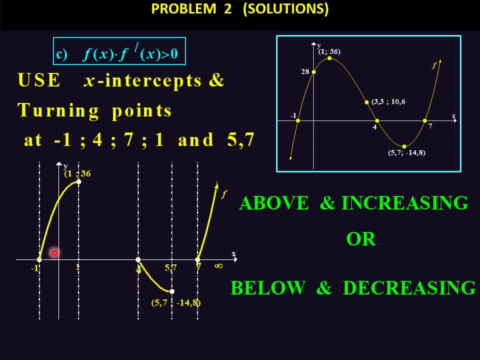 this portion is below and it's decreasing. so there's three intervals, so there's quite. you see, try to sort out that- and you can see. there's it's above and inc. you can just focus on the above. there's the above and that was the increasing part of the above. 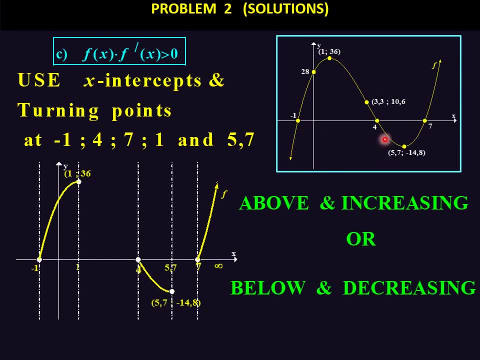 which is that portion here, there's the below and that is the decreasing part, and then we can just read off the intervals from there. okay, there's it from negative one to one, and this is from four to five comma seven, and that's from seven up to. 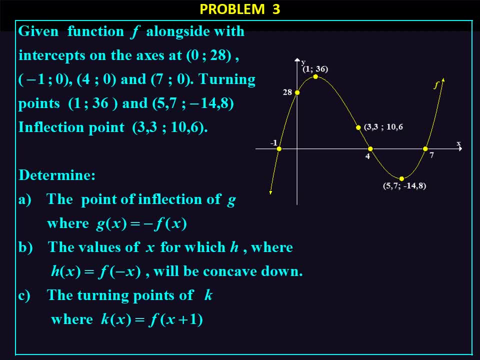 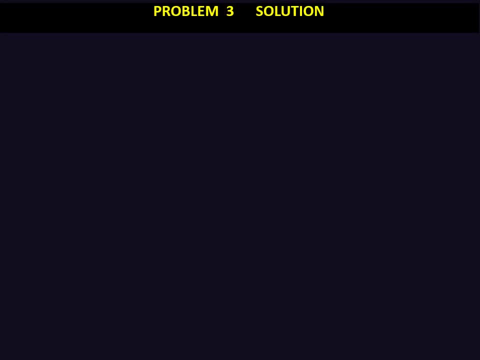 let's look at the third problem. here we're taking the same graph, but we have- we just have different questions on it- the point of inflection of g, but this was the f graph. what do they say is g? so there's that. so let's look at questions here. the point of inflection, so i need to. there's my point of. 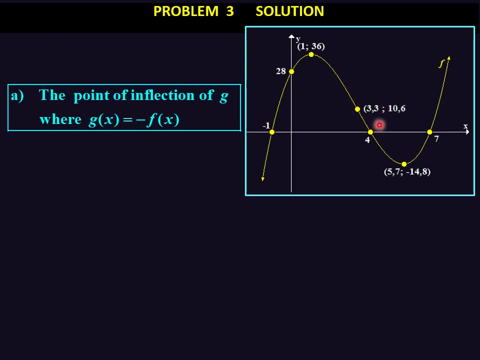 inflection- but this is the point of inflection- of f at x equal to three comma three. but now, now they have a new function defined by gx, equal to negative fx. what is negative fx mean that that's correct. that means the graph is reflected in the. so that's the original inflection. 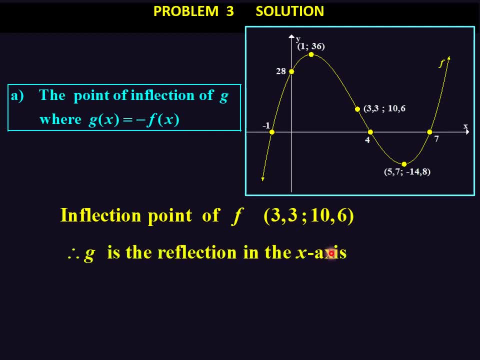 point. but we want to get the reflection in the x-axis right. so reflection in the x-axis means that that one will stay a one, but that 36 become a negative 36 right and that 5, 7 stays. it's the y values that change. 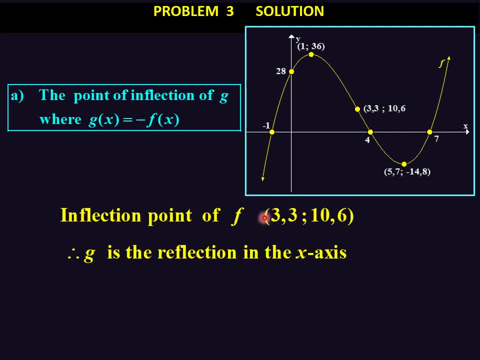 so if i reflect that in the, so the x value is going to remain the same. it's the y value that when you reflect in the x-axis, the x coordinate remains the same. so we just change the 10 comma 6 to negative 10 comma 6.. 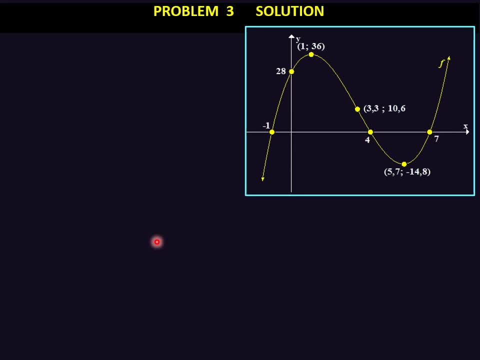 let's look at the second question in this problem. there's the graph. let's look at the question. the values of x, for which h will be concave, b down and their h. is this defined this way? what does f negative x mean? that's correct. it means: 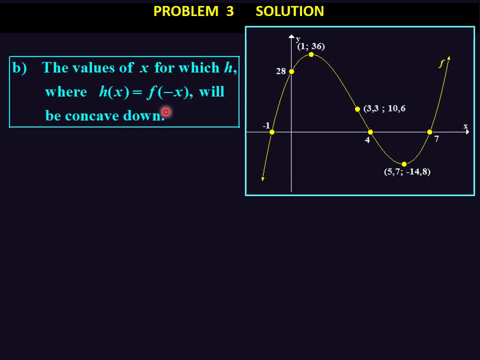 where the graph, the, the f curve, must be reflected in the y-axis. okay, concave down. the original one is concave down. there's a concave down from negative infinity to three comma three. but h is the reflection in the y-axis. let's just reflect it in the y-axis. 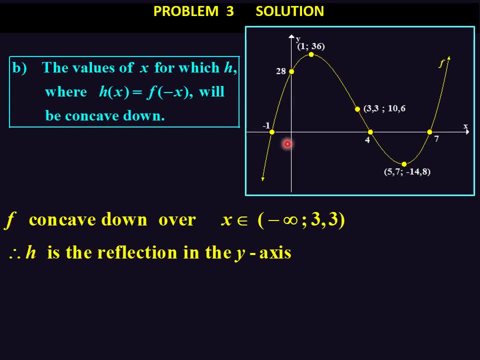 so, in other words, this point will go this way, that one will go that way. so let's just see, there there's. this is what the reflection looks like, and now can you see where's the concave down. now, concave down. you see, their concave down was on the left side. here concave down is on the right. 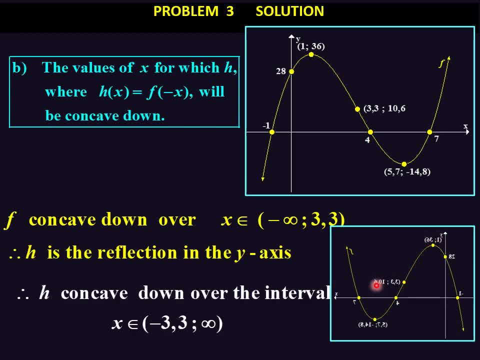 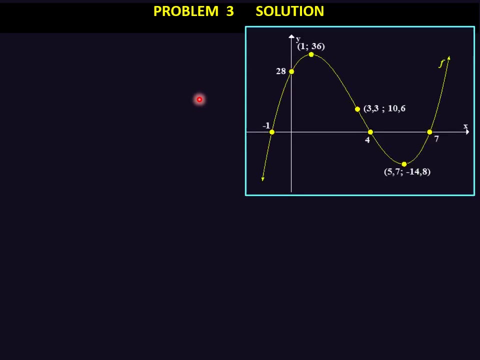 side. so it's from this point and that point is from negative three comma three, see from negative three comma three up to infinity. let's look at the third question in this of this problem: determine the turning points of k and their kx is defined as kx equal to fx plus 1. okay, let's see what we mean by that turning. 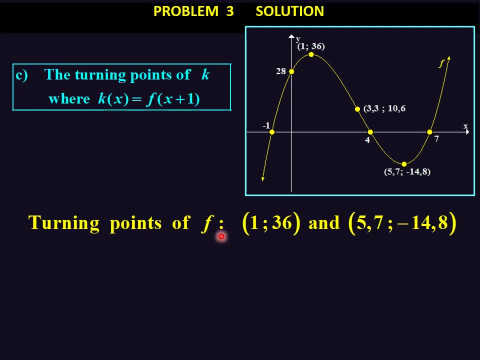 points. what are the turning points of f? those are the turning points. we can read it off from our graph. but now, x plus one. what does that mean? when you have x plus one, you can read it well, see if it is true or not. that's correct. the graph is shifted. one unit plus one means one unit to the left. 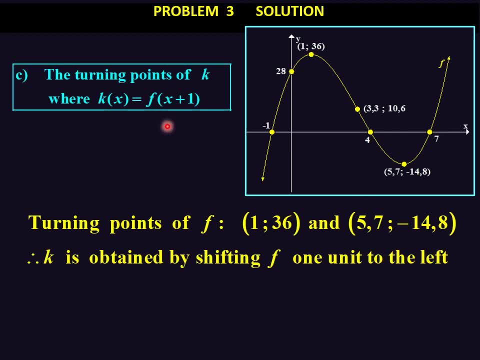 there. if it's negative subtract one, it means to the right, but positive one is one unit to the left. so I must take one unit to the left. so which coordinate is going to change? that's correct, the X coordinate there. so it's one subtract one which gives me zero. the other one, these five comma seven, subtract one that gives 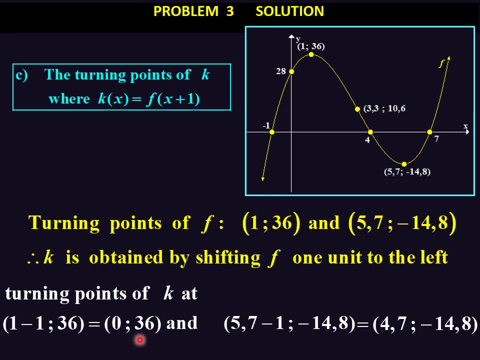 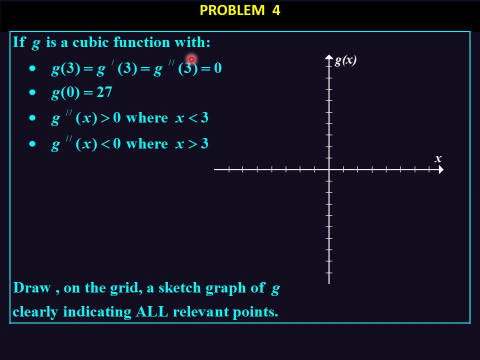 me four comma seven. so these zero and thirty six and four comma seven negative fourteen comma eight, that those are the turning points of the new function. let's look at the fourth problem now. if G is a cubic function, so they have a cubic function. it's not drawn G, X or all these. this is all the. 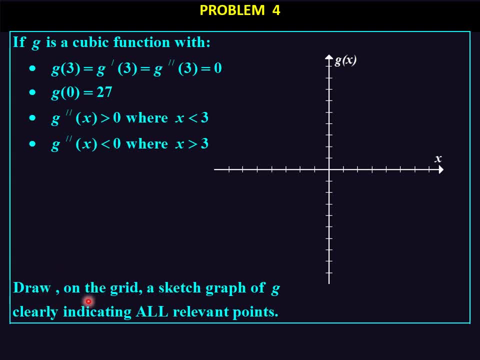 information that's going to be given to us in the next section of this video. so we're going to try to interpret this. so you must. there's no equation given. there are some statements here: G 3 equal to G, prime 3 equal to G, double prime 3 equal. 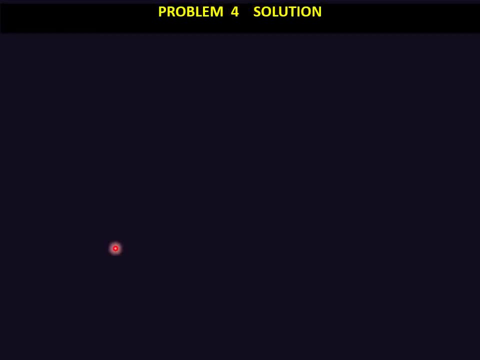 to zero. let's, let's use the given information: G, 3 equal to zero. what does that mean? X is equal to 3 and Y equal to zero. that is, an X intercept at 3: 0. let's plot that point in the meantime, and there we. 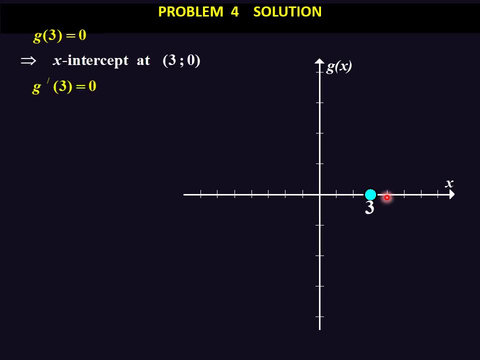 have the point there. let's look at the other given information: first derivative substituting 3 equal to 0. so there we have. X is equal to 3, but first derivative mean there that I have a turning, or so I have a critical value at 3, so there's a. 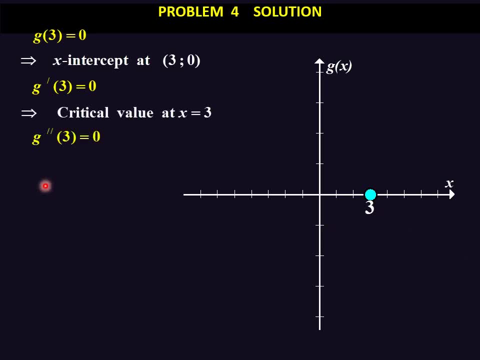 critical value here. then we have the second derivative, 3 equal to 0, and then second derivative. that means that I have an inflection right. so we have an inflection point at X equal to 3. so this is actually not a maximum or a minimum, it's actually an inflection. 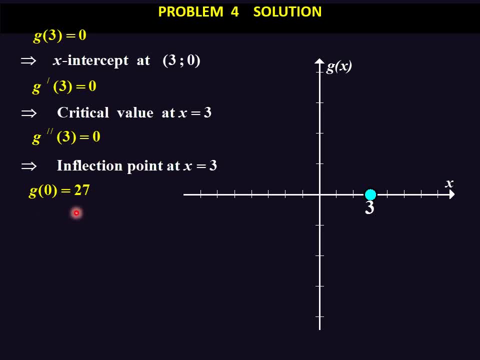 G 0 equal to 27. that means X is 0, Y is 27. that is a Y intercept. let's plot the Y intercept and there we have the Y intercept. then we have second derivative X greater than zero. but X must be less than 3. so on the left side of 3, what does this mean? second derivative greater. 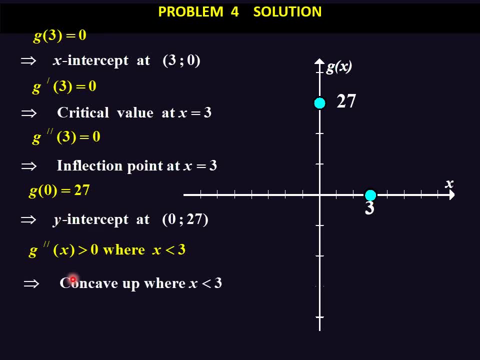 than zero. that's correct. that means I have concavity, so it's concave up. so on this side will be concave up. and which way is concave up? let's see, there is concave up. then we take second derivative less than 0. second derivative less than zero, that implies I've got concave down. so let's see. 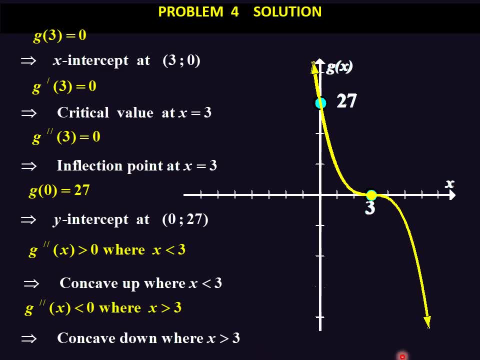 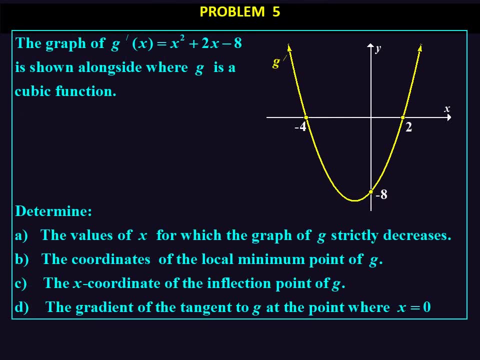 down, and there we have concave down, and there we have our function. let's look at problem number five. here we have the following: given information, we have a graph of a first derivative quadratic there and there's the graph of the first derivative right, and then we have some questions based on this graph. 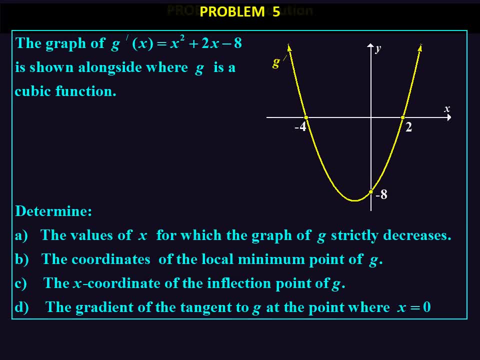 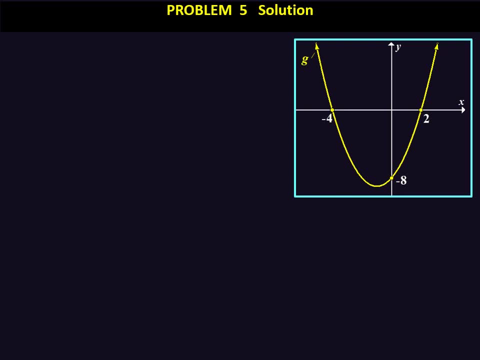 of the first derivative. let's look at each of the sub questions. now there's the graph of the first derivative as given: determine the values of X, for which the graph of G will be strictly increasing. is this the graph of G? no, this is the graph of the first derivative, but the graph of G decreases is the first. 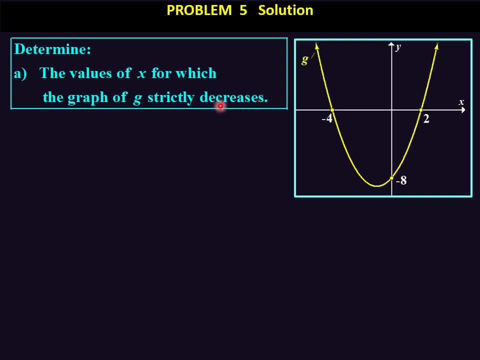 derivative of the first derivative is less than zero. so where's the first derivative here? less than zero. so that's what we need to do. first derivative less than zero. it's below the x-axis. you see, below the x-axis there is the first derivative and that is between negative. 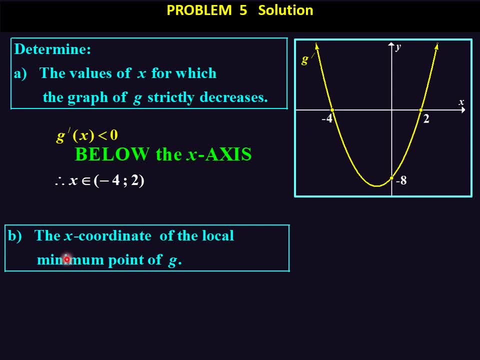 four and two. let's look at the second question. we must find the X coordinate of the local minimum point. now, local minimum would be where the the local minimum would be where the gradient changes from negative to positive. let's see now: there the gradient is positive and then negative. so this is not a local minimum. here the 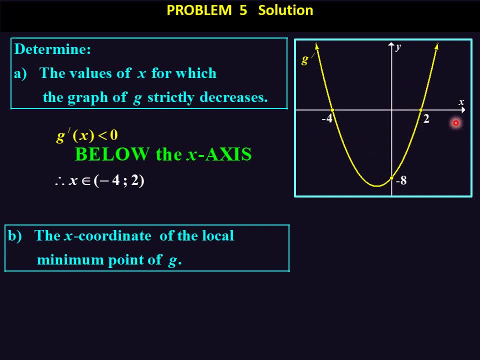 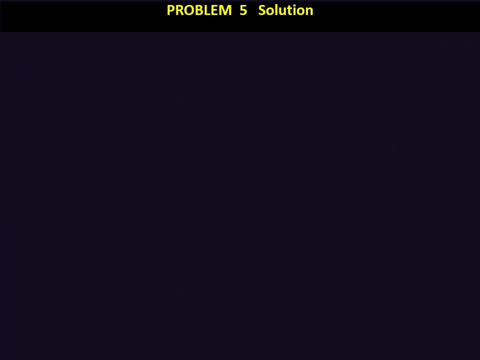 gradient is negative and then it becomes, but so this is where we'll get a local minimum. right changes from negative to positive. there is negative and then positive. therefore, we have a local minimum at X equal to two. let's look at the next one. we want to find the X coordinate of the inflection. 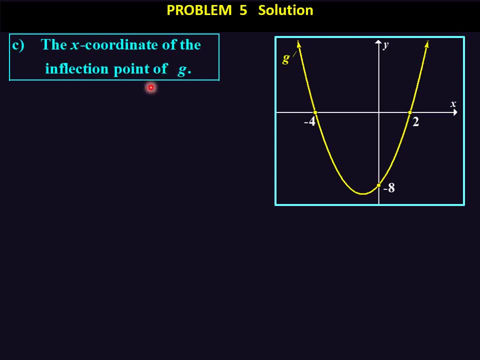 point right, the inflection point of G would be the second derivative right. but now we have the first derivative there. so the inflection point if this, if the first derivative is a quadratic, the inflection point would be between those two x intercepts there, so between them, exactly in the middle. how do we find that we add the two? 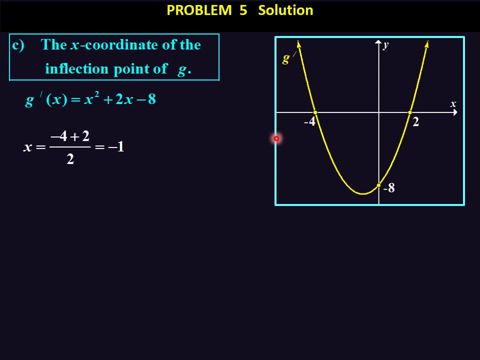 negative four plus two, then we divide it by two and that gives us negative one. or if this is the first derivative that's given for inflection point, you just find the second derivative, so let's differentiate that. that gives us two. x plus two equated to zero. solve for x. 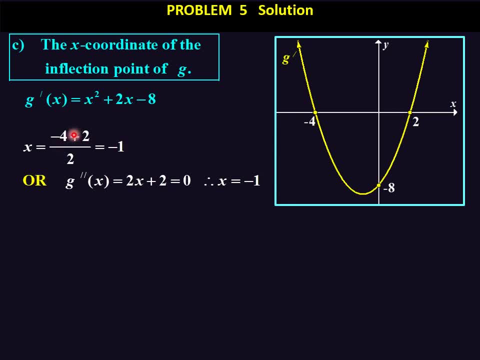 and we get exactly the same answer there. you can either find the inflection, which is the midpoint between the two x-intercepts, or you can actually calculate the second derivative and equated to zero. let's look at the following question. we must find the gradient of the tangent gradient. 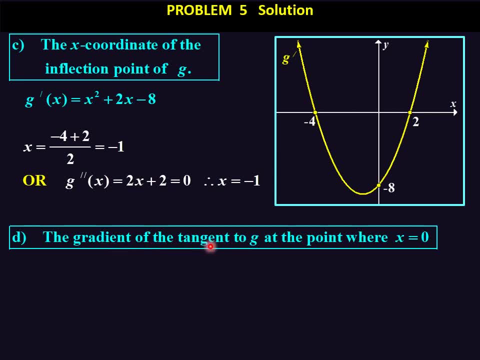 of the tangent is the first derivative. so actually we can use the first derivative. so the first derivative is the first derivative. so the first derivative is the first derivative. derivative is actually the graph where x is zero. so if i make x is zero here i end up with negative. 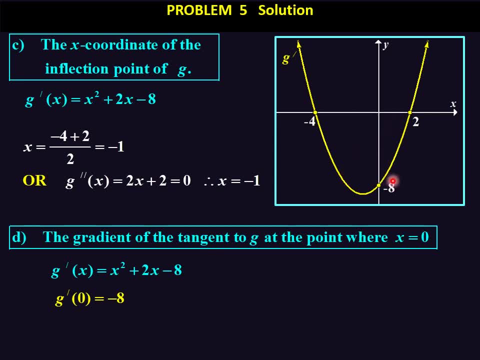 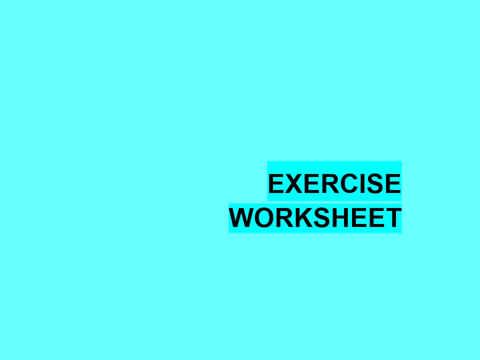 eight, or i can actually look there. if there's zero there's, then i can actually read it also. there's x zero and it corresponds with negative eight. so the gradient here, in this case m, is equal to negative eight. before we actually start with the x general derivative, we'll say negative h is 0, because we already know in this discussion. 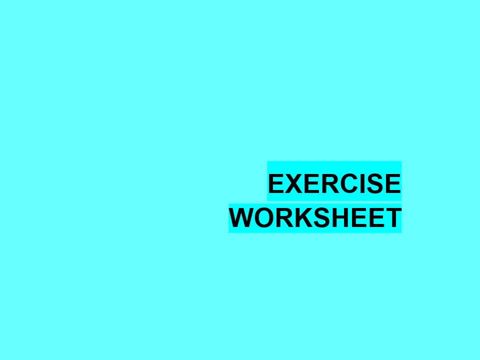 we know that it isasha zero and negative h. remember 96% is the base of the base of h. we also said, when we use the binaryül, the x of h is 0 due to an index at the 6th number. after that, twenty zero makes negative three. zero, which is times negative four. 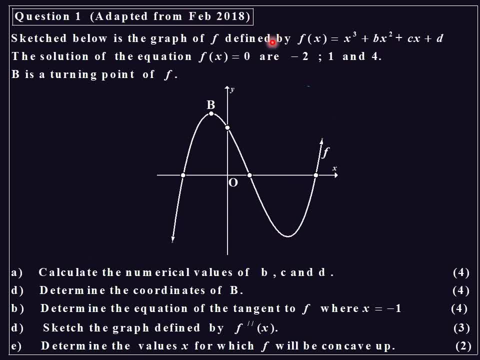 delta, prime. those is 믿습니다 that say guilty zero, not negative zero, and finally give your limit immediate zero, adapted from external DBE question papers there. so there, we have a given information and they ask you to work out the values of b, c and d. you see the b? c at three unknowns, so they need to. 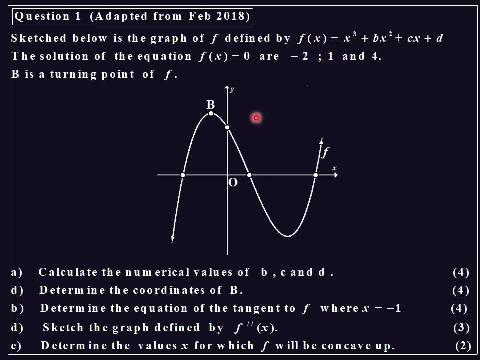 give me three. and there we've got three points there already, right then they want the coordinates of b. what is b? the coordinates of the turning point. we want the equation of a tangent. then we must sketch the. what must we sketch here? you must sketch the second derivative and the second. 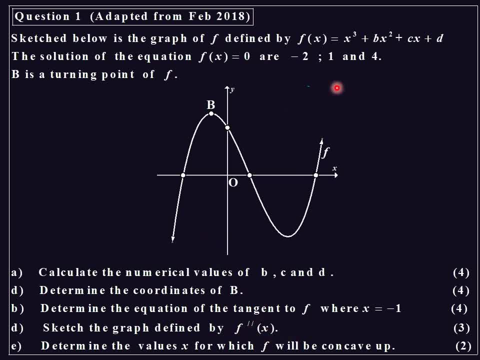 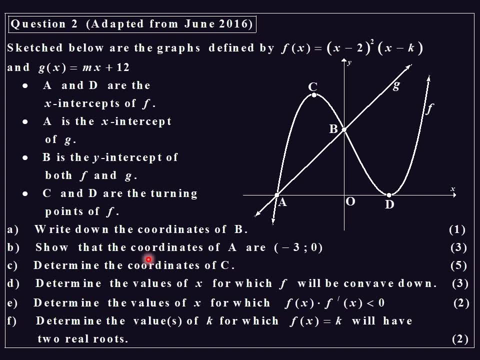 derivative of a cubic is. can you still remember that? that's correct? it's a linear function and here you want to know where is it concave up? and we have a similar type of situation here. there's some given information and some questions there. there we even have one similar to what we 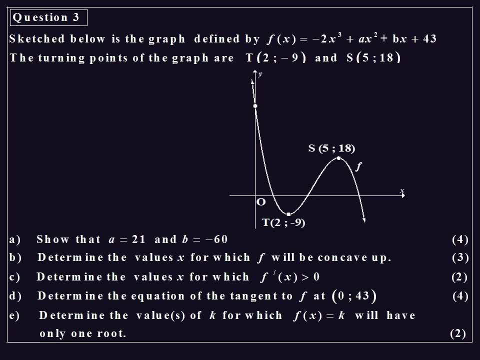 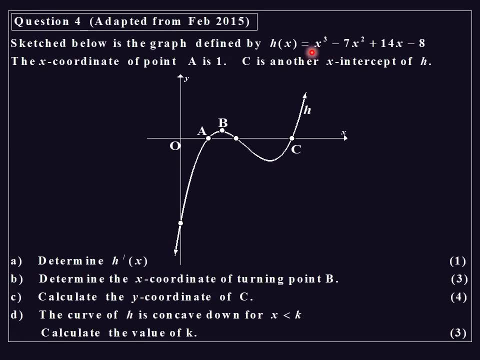 did earlier, and then there are some more questions. there we've got two turning points. you can see what we need to do there. there's another one and we have different questions based on that. there the equation is given, the graph is sketched and there are some questions. 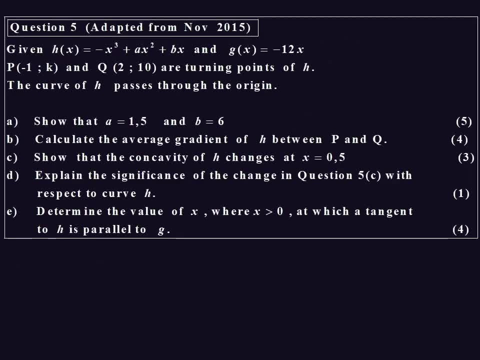 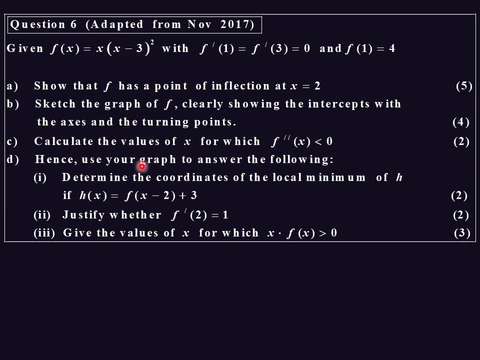 then you have to do some interpretation as well. same applies to question number five. here we have average gradient. that's average gradient. some of the work we did in part two, yeah, it's just a different form. and here they also want you to see what you need to do in order to get to the 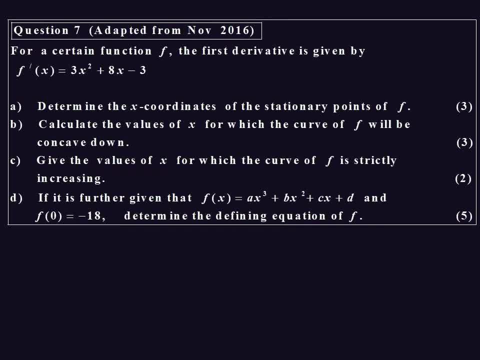 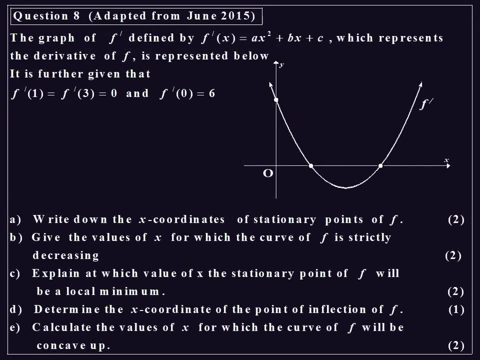 question number five: here we have average gradient, some of the work we did in part two. yeah, it's just a sketch, the graph. question number seven: there the first derivative is given something similar to the last question. let's look at this question here. this is the last question. question eight: 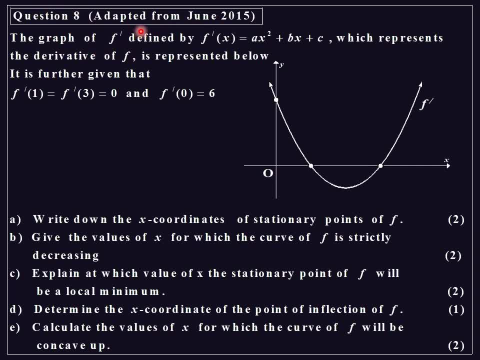 it's adapted from the june 2015 paper. here we have the graph of a first derivative. there's the first derivative and we tell you: the first derivative at one and the first derivative at three. they are both equal to zero. so we have the first derivative at one and the first derivative.